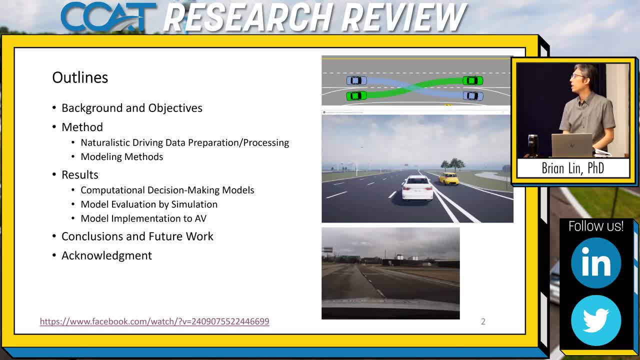 objectives and then share with you what method we have applied and some results, also the conclusion and future work. So if you see the three pictures on the right, so these are basically the three, you know, main topics we would like to cover in the presentation today. So first we would like to understand what is the weaving 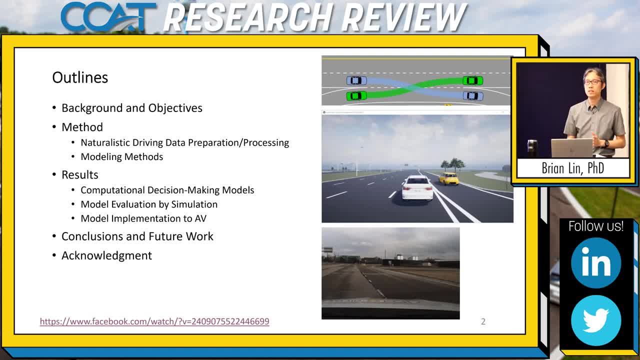 section and what driver's decision making, why it's important in the weaving section. And then the second picture shows that the computer simulation we ran with Simulink and then we further tested to create a demonstration scenario in the MCITI test facility with the real automated 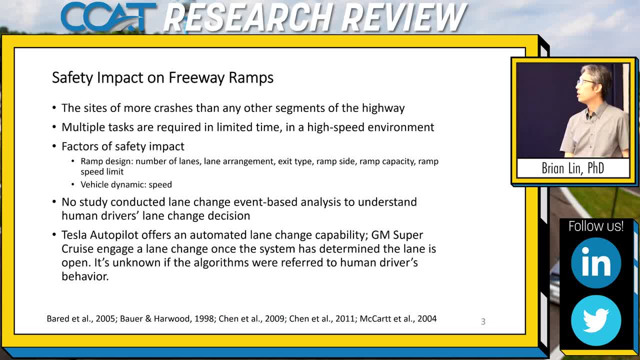 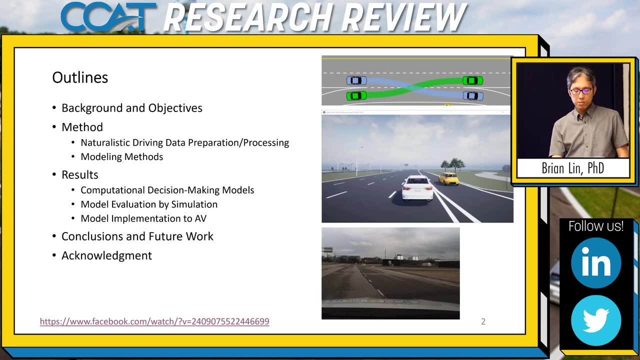 vehicle. So before we start digging into our, you know sharing the findings in our in this study, so we'll first like to. I'll go back to the previous page. So before we talk more about this study, I would like to share with you a video about the weaving. 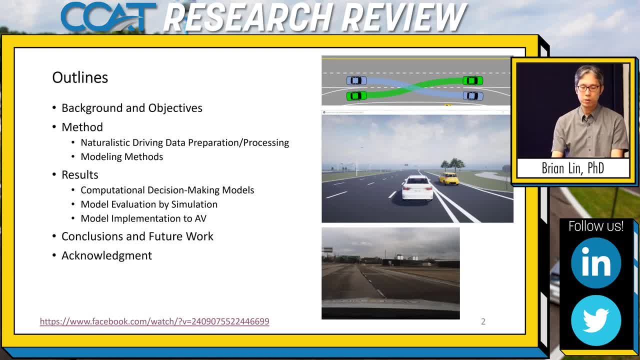 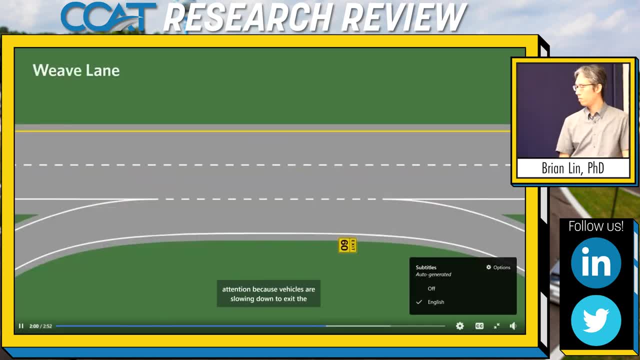 sections and how you know, drivers will interact with the other vehicles. in the weaving section, The weave or crossover lane requires a driver's full attention because vehicles are slowing down to exit the highway while other vehicles are speeding up to enter. It's important to control your speed and the timing of your lane change. 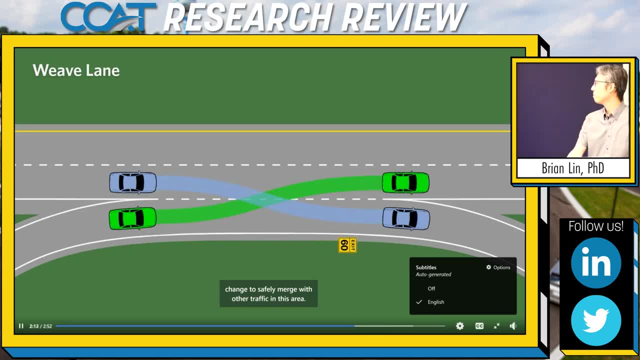 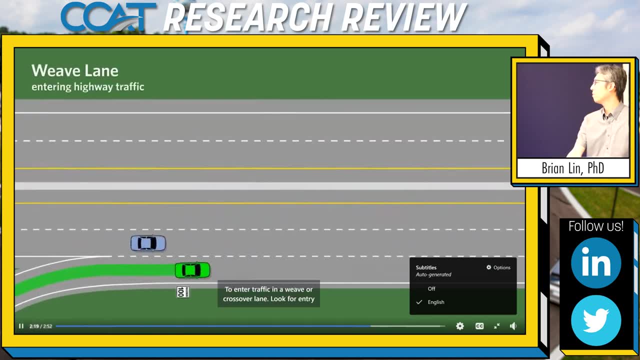 to safely merge with other traffic in this area. To enter traffic in a weave or crossover lane. look for entry space in traffic and accelerate to traffic speed. Shoulder check to look for speed. Adjust speed. to look for exit space. to enter traffic again. 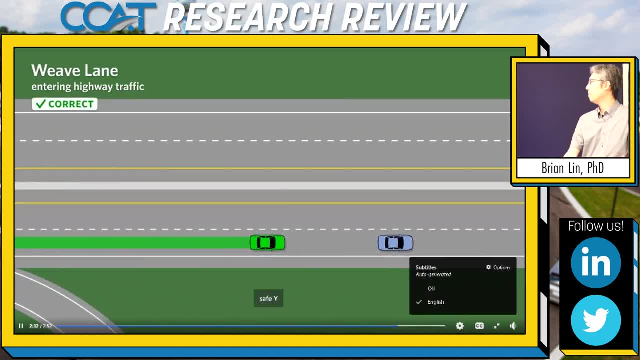 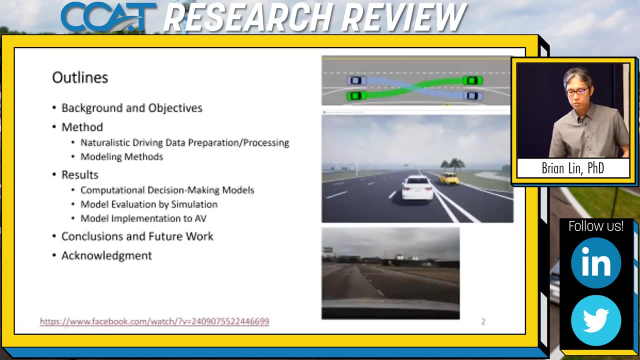 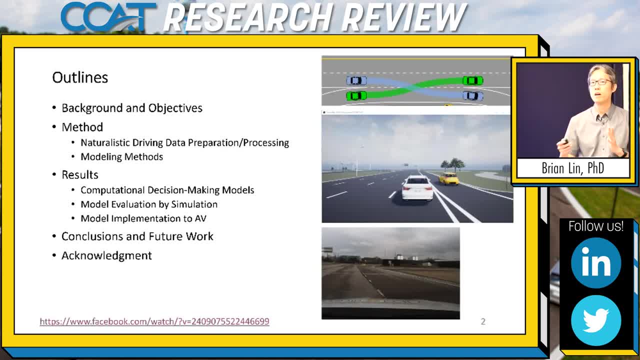 The vehicle is moving, but the vehicle is not moving. You know, in the real world the length of the weaving section is that you know that it's varied, So it could be very long, could be very short, So driver has to respond to. 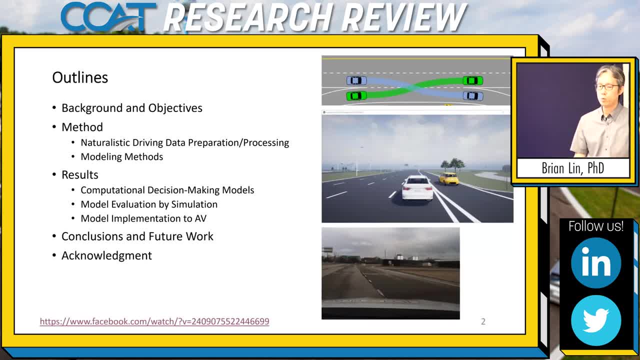 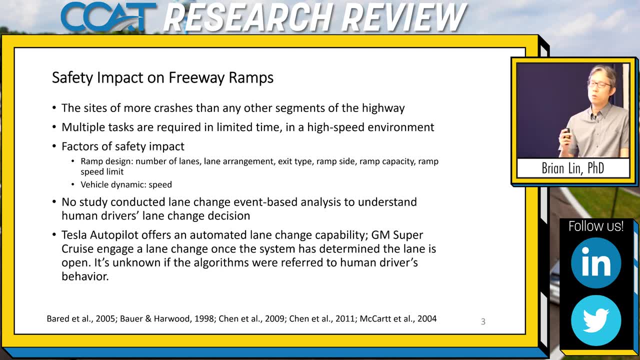 and the other vehicles maneuver in a limited length of the weaving sections. So that's why, as a safety impact on the freeway ramps, well, the weaving section, the site, has more crashes than any other segments of the highway And, as I just mentioned, the driver. 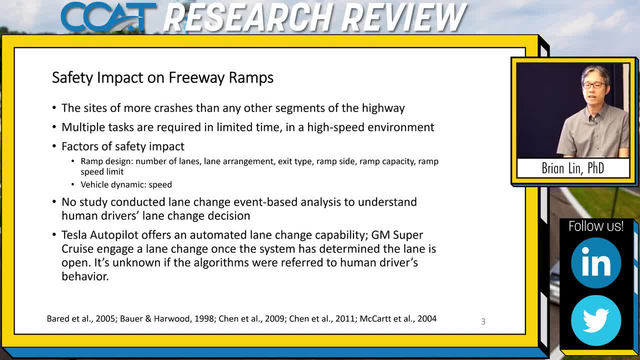 needs to engage with multiple tasks in a very limited time And especially it depends on how fast they drove And it could be- they need to, you know, process multiple tasks within only like five to 10 seconds, And then and also, they need to keep the driving environment safe. 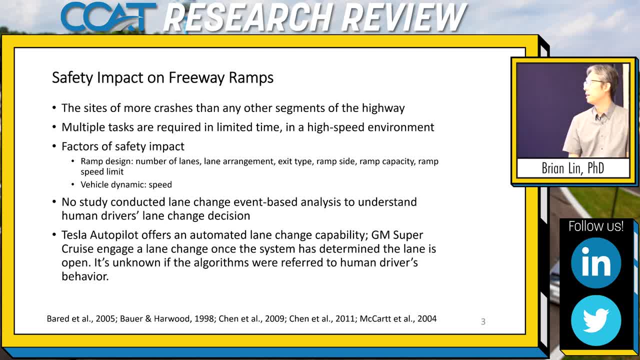 So from the previous literature mentioned about the, the factors of the safety impact. So we want to care about the ramp design which is in this study. we we especially focus on the weaving sections. That's the very special design on the, on the as the regular ramp, And we also need to care about the vehicle dynamic. 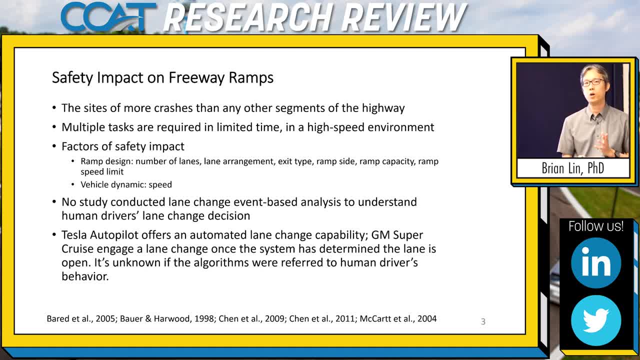 The speed here includes the drive, Well, the whole ego, vehicle speed and also the other road users speed. So, as the animation just mentioned, you have to control your speed in a good way and interact with the other road users And either speed up or slow down to before you merge into the target lane. 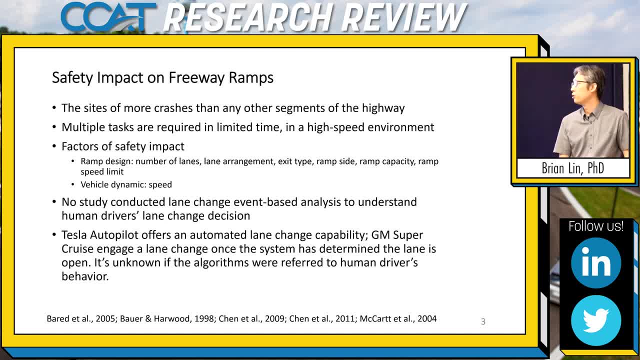 So so far no study had a conduct had conducted lane change event based analysis to understand human driver's lane change position. Here we focus, we want to, you know, we want to emphasize the human driver's lane change decision. The real reason is: 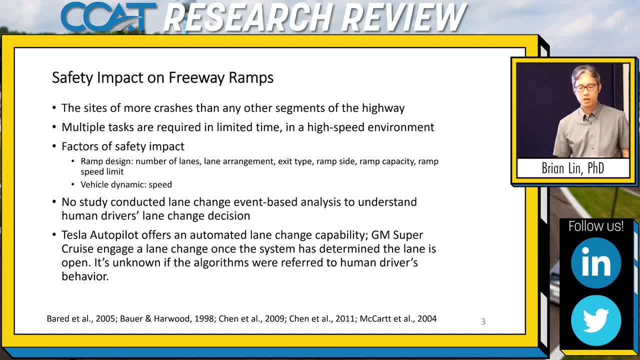 when we try to develop the autonomous vehicles. autonomous vehicle features well understanding um the human driver behavior is important since we want to make sure the maneuver and all the decision-making from the automated vehicles will meet the the uh expectation of the human. 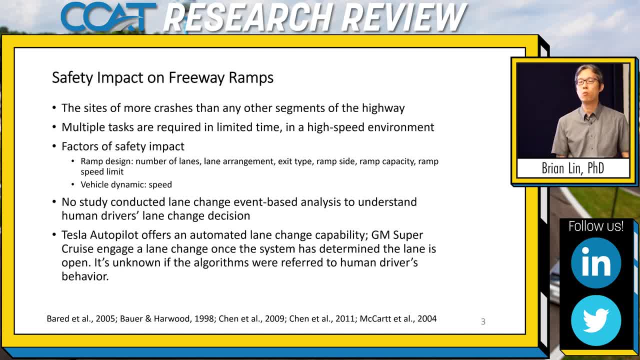 drivers, And so human driver, will not feel confused. that why the vehicle performed this way. So they may want to override or, you know, feel very confused, feel confused about what the vehicle is doing. So so far, tesla autopilot. 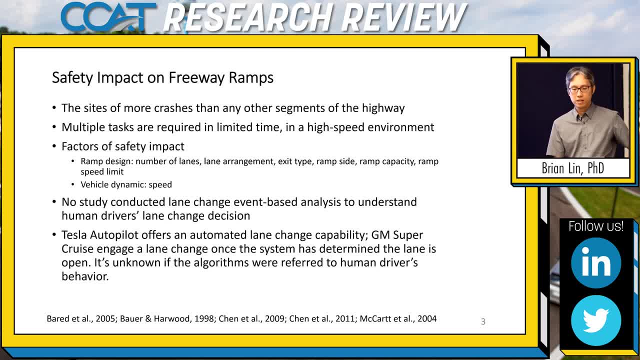 they offer? they offer the automated main chain capacity compatibility, and gm super cruise has that as well. but it's unknown if their algorithms or models were referred to human drivers behavior. so in this study we further like to, you know, create from the bottom up, like the bottom up. 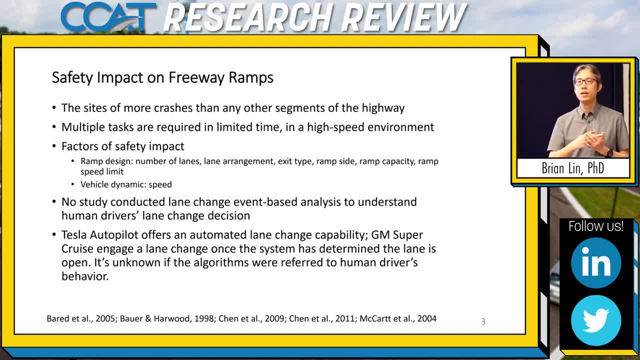 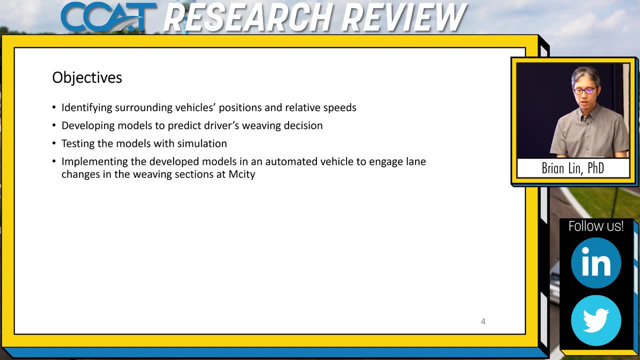 we started from the data and we validate the data in the simulation environment and then we create, we further implement such models into the in the real world, on the test track and to see how that works. so there are four objectives and which are the four major tasks in this study. so first we 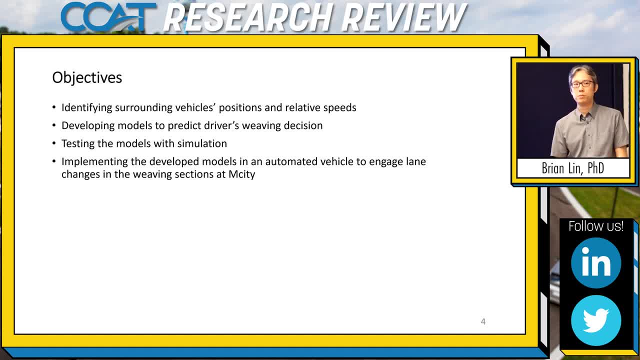 need to identify the surrounding vehicle's position around the speeds using the or the naturalistic data we have, and then we'll develop the models for the weaving decision. so here we focus on the decision itself. so the simply said it's going to be a for, a go or a no-go. so the weaving decision. 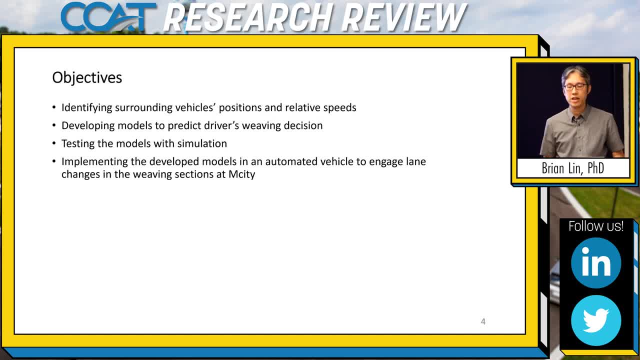 they want to merge to the target lane or stay in the original. but in other words, if they stay in the original lane, you know before they, before the weaving section has been run out, and they will miss this exit or entrance. and with the developed models we further tested with a 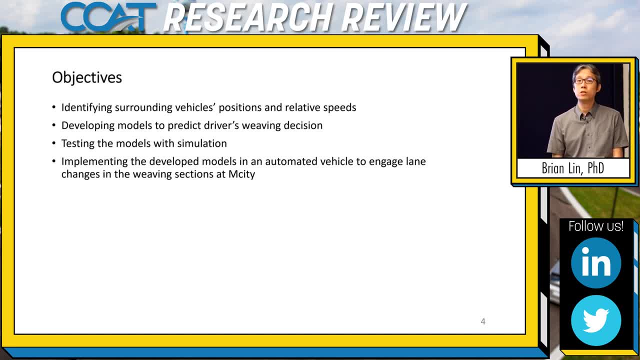 computer system to see how that works in the simulation. so i'll share in this presentation today. i'll share with you some 3d simulation we created using the simulink and also with some with some performance measures to see how that works in the simulation and then we further implement that in the 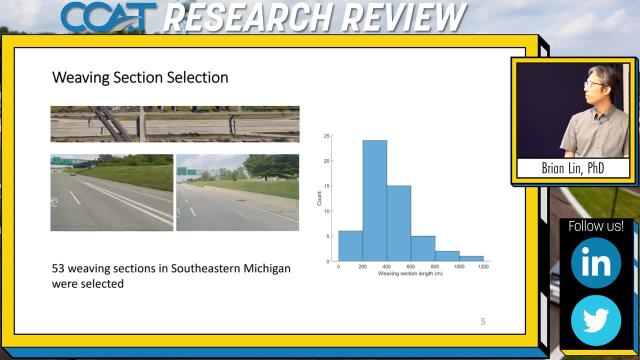 weaving section at m-city test facilities. so for before we extracted the data from the naturalistic database, we first need to select the the weaving sections, the candidate of the weaving section. so totally, we selected 53 weaving sections in southeastern michigan and he, here are the um, the 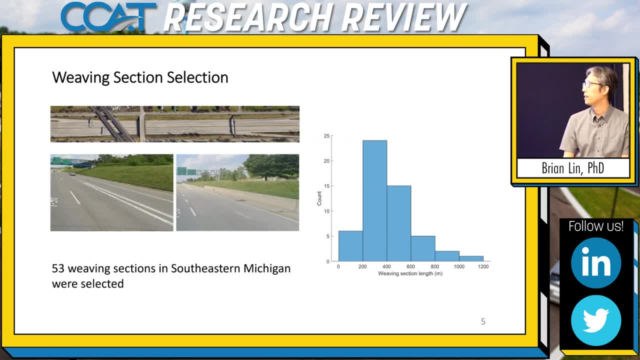 pictures, as the typical one on interstate 96 around the metro detroit area. so you can from um in this. in the picture on the top you can see it's. it's kind of a relatively long weaving sections so it's about like 800 meters to um 1000 meter, but it's not always this long. so if you see the 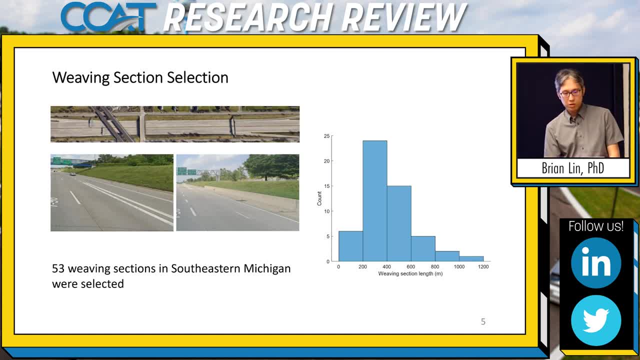 distribution on the rise. in the histogram you will see some of these are shorter than 200 meters and most of them are between 200 and 400 meters and some- you know, but you know most of that will be um- has the length between 200 and 600.. 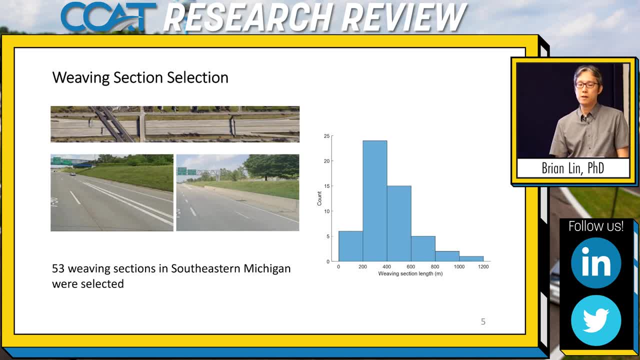 in other words, if you drive with a speed of um, let's say, 75 miles per hour, and then you will, and if the weaving section is about 300 meters, you will run out the weaving section within 10 seconds. so you don't have much time to respond and you don't have much time to make the decision. 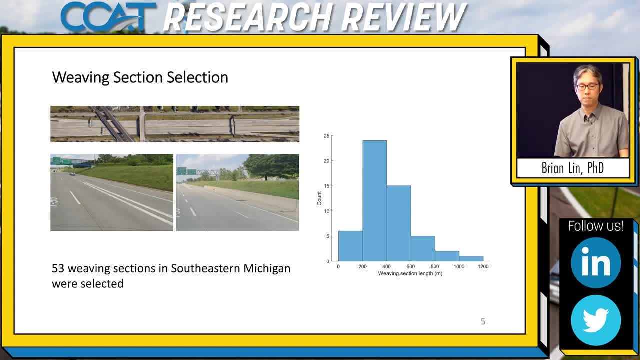 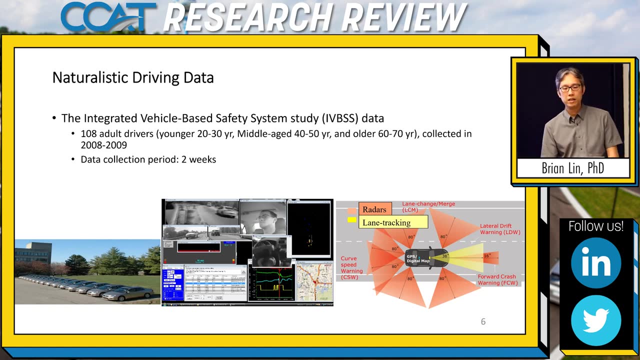 so i have to, you know, with the, the assist from the um automated vehicles, that will, uh, give you some. you know, that's a very important assistance for the human drivers. so next i would like to talk about the naturalistic data and some of the attendants. 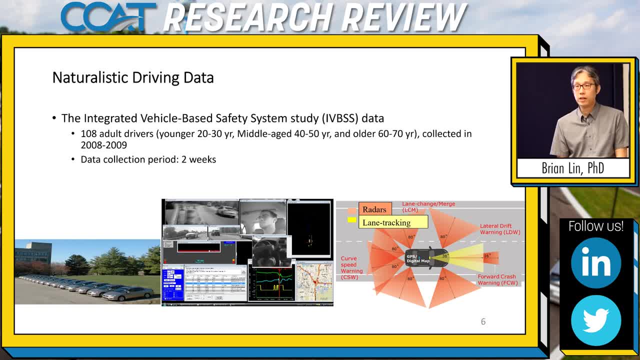 were familiar with this data sets. we have been used, widely used in umtree researchers. so totally in this ibbs data sets we have 108 drivers- adult drivers- so evenly distributed in three age groups and collected in between 2008 and 2009.. so for each subject, the data collection period is about two weeks and for the um, for each vehicle. 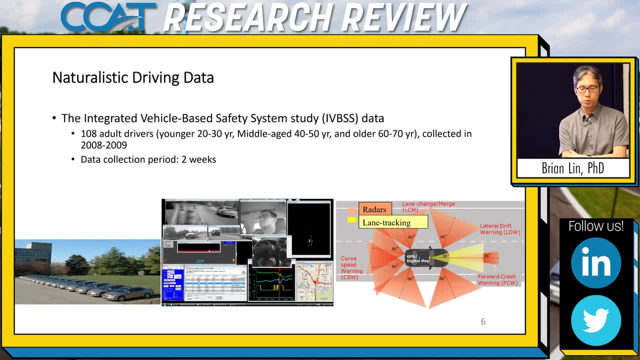 um, the the drivers own for the during the two weeks. uh, we have the. we have six radars. well, seven radar sensors installed, um, you know, facing two different angles, and to the um to the external world. so, if you see the plots on the bottom right corner, so each um, you know, you can see that there's. 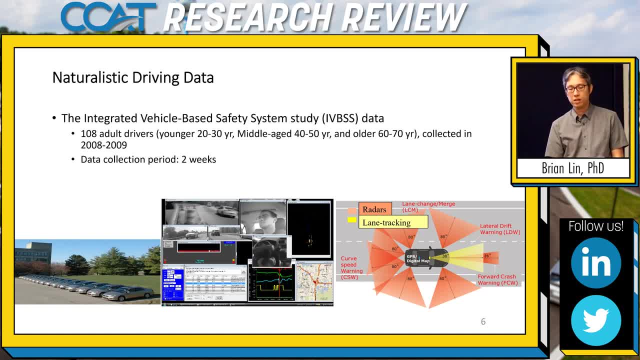 a very large um. each orange triangles means the the the field of view of the short-range radar sensors. it covers um 150 degrees field of view and 30 meters of the range. so we rely on those radar sensors to tell us who is driving next to the eagle vehicle and how fast they're driving. 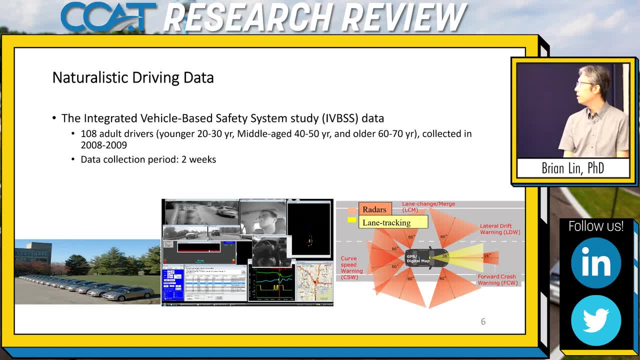 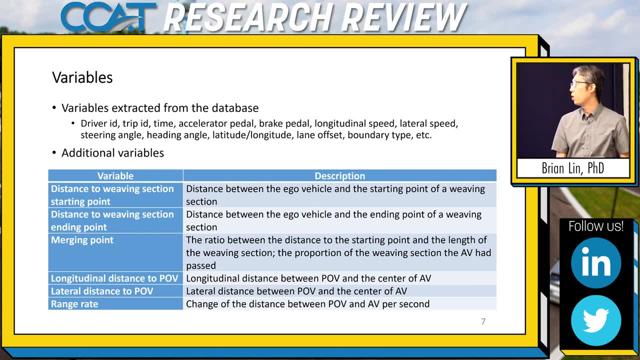 and also what they're doing next. So about the variables we extracted from the database, I will not walk through that. I listed some examples here And the more important is the additional variables listed in the table at the bottom. So these variables were kind of what we extracted, we processed from the extracted data and also from the map. 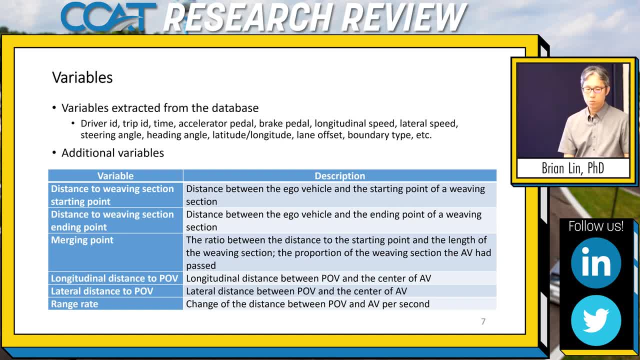 So the first, well, the first two, the first three variables are very important and I'll share with your findings and later the presentation. So this is about the distance to the weaving section- starting point and ending point- And also we convert that these two numbers into a merging point as a percentage or as a ratio. 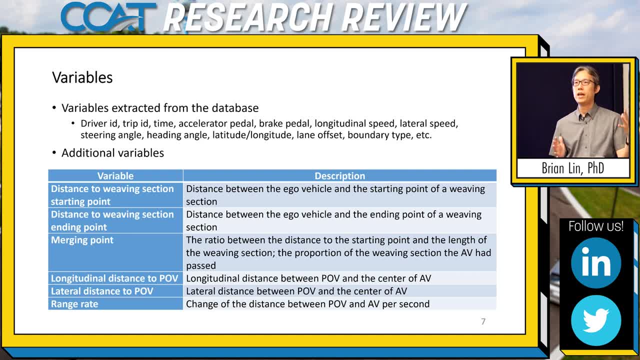 So, for example, if we have a 800. Length of the weaving section at 800 meters And if the driver decided to merge on to the, you know 400 meters after the starting point and the merging point will be point five, 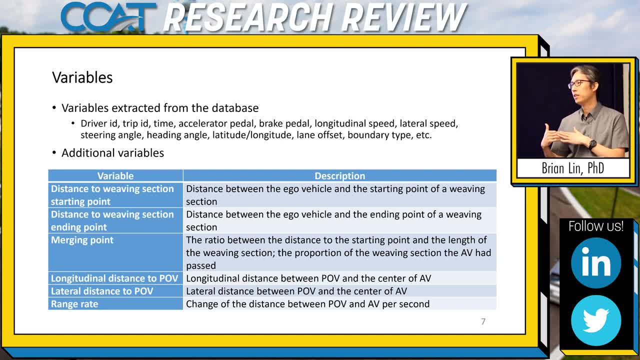 And the distance to the weaving section, starting point will be 400 meter and 400, another 400 meter to the ending point. So this is important, since we would like to know at what, at what position, the driver started to merge And, And you know, sometimes it may not be related to safety, but related to they have to, Otherwise they will miss this exit or entrance. 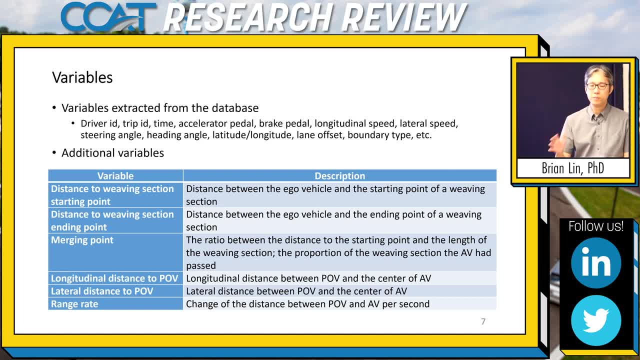 And on the other hand we would like to also need the, you know the, the association with the other vehicles. so here we use the POV, which is the private owned vehicles, as the abbreviate abbreviation. So we need the longitudinal distance to that lateral distance and also the range. 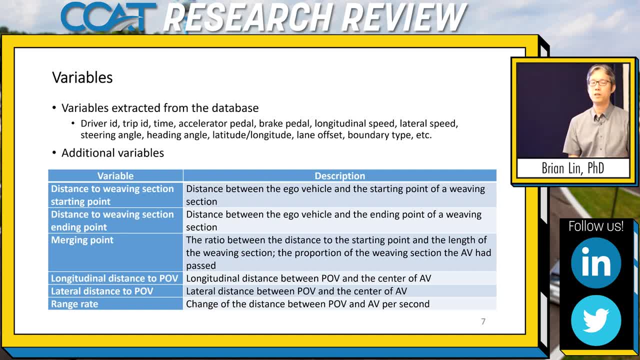 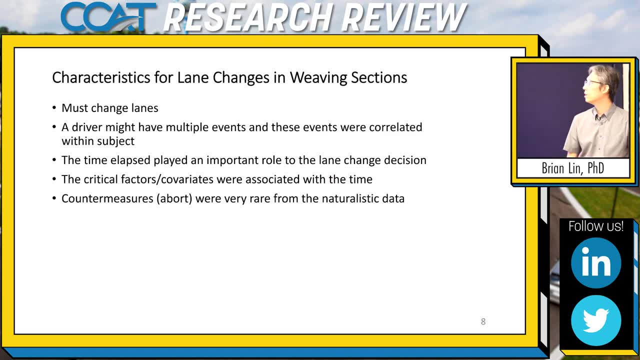 The bulunance that doesn't look like it but has a top line design, eithericus design, Oh hardenings and also range rate. So these three are basically what we want to know: where the other vehicle is and what they were doing. 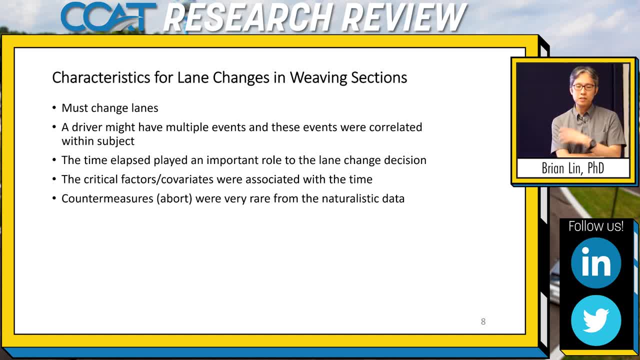 Okay, So Here I listed several characteristics. when we, you know, when we analyze the dataset from the naturalistic data thing that's, this is a very different scenarios as we see from the, you know, discretionary lane changes or the lane changes in different areas on the highway. so first, the most important thing. 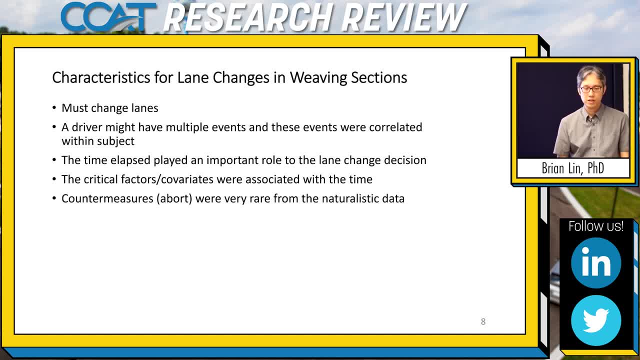 the driver must make a lane change. it's a must for, and all of the drivers, including you and me, we will select to do so. even it's a very risky situation. we get very close. you know we have a. you know we have a very large range way to the other road users, but we will try our best to make. 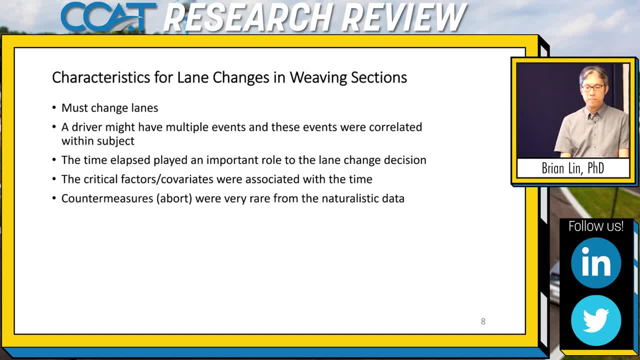 this lane change and go to our target lane. and the other thing is the driver will have multiple events. well, each driver will have multiple events and these events were correlated to within the subject. so that's from the data side. you know some subjects. they may have one event and some. 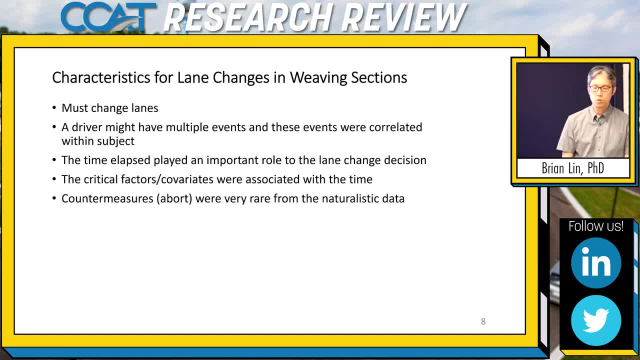 subjects may have multiple, more than 10, so we will have to treat the data from each driver as the as a correlated to each other. so, and we also found that the time elapsed played an important role to the lane change decision. so, based on these characteristics of the lane changes, 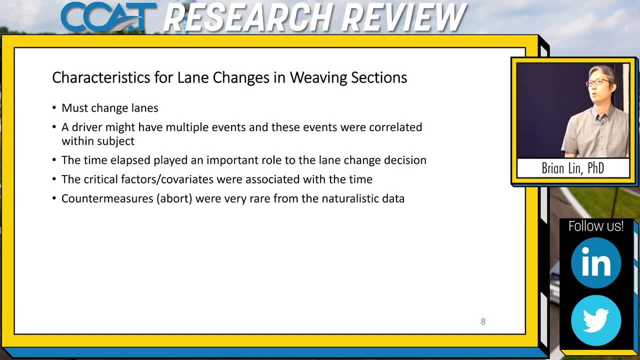 we selected. originally we proposed to use some machine learning methods, but after that we found that it was not very, you know, appropriate of using that, because these reasons, because of these reasons and the critic and also the critical factors and the covariates were associated with the time, so, in other words, as the time being the, that's, for example, as time being the merging, 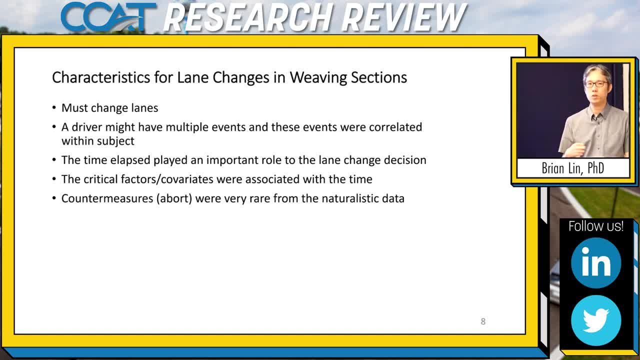 position will be more and more important, since the longer you stay in the eagle lane, the shorter weaving section to the end of shorter distance to the end of a weaving section you will have. so you have to. you know this factor will become more and more critical as time, and so we have to use some other techniques to analyze. 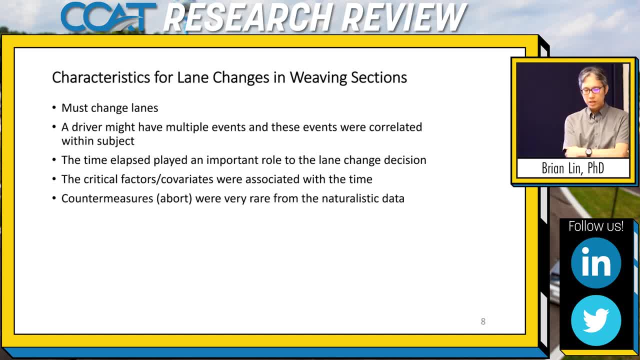 the data and to to do the modeling and also, uh, from the naturalist data. it's very difficult for and very rare cases as the countermeasures, like the abort of the um or of the lane, change, as i mentioned, all of the drivers. they will try to do their best to merge onto the highway or to take 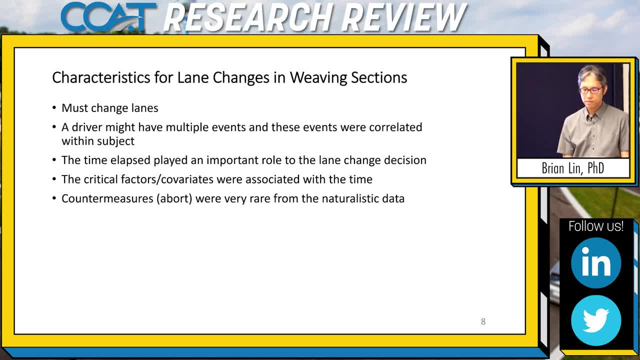 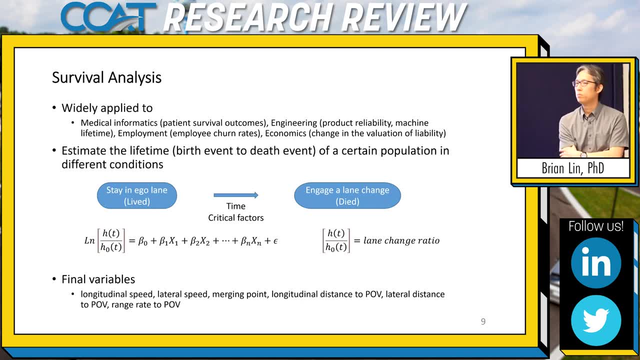 the exit. so here's the method we applied: um to. you know, replace the machine learning methods. so it's a survival analysis. it's being widely used in the medical department and it's a survival analysis. it's being widely used in the medical department and it's a survival analysis. it's being widely used in the medical department. 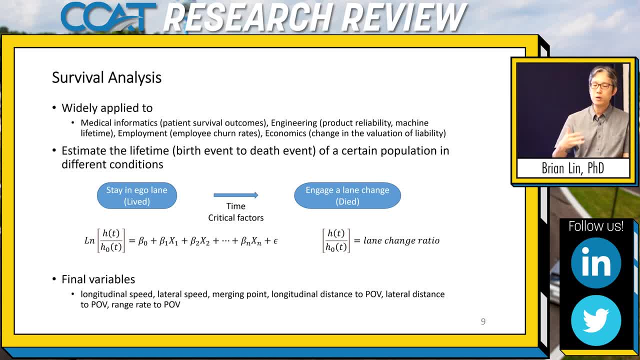 for you know, for example, in the medical, informatics, engineering, employment, economics, and you know that they try to estimate a lifetime uh from the certain pep of the certain population, different conditions. so in other words, if we try to under estimate how long um this machine can can work. 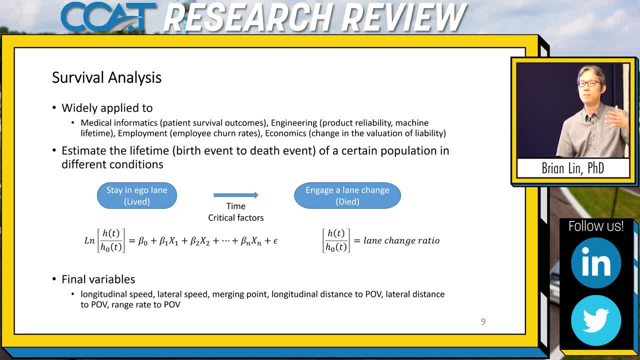 before it's it's it's been broken so you can start. you know from this, you know this. the startup is working and then estimate at maybe three months after: uh, it has the performance lower than what's lower than 50 and after another three months it dropped. 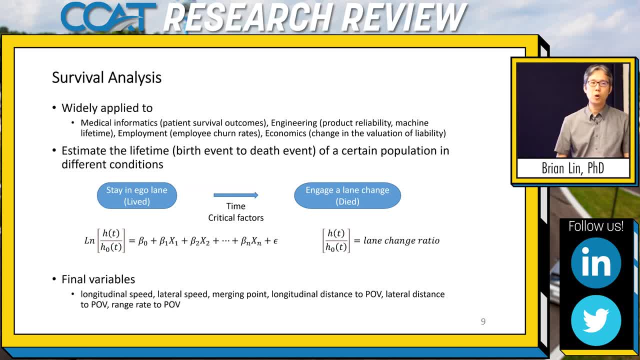 to 25 and another three months it died. so use this kind of um survival analysis to to make sure to observe at what time the? um the events will occur and before that um the all of the other events will re. well, the remain. the events will remain as it was, and then at a single specific time. 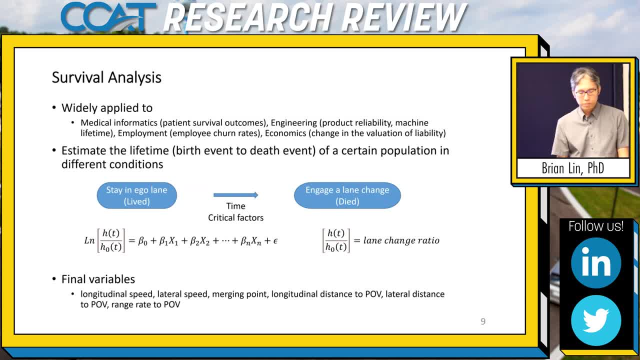 it died, or we say the event occurred. so in this study- um well, you should see in the like the illustration in the middle. so in this study, our live event. it's just like you know, the drivers stay in the eagle lane, so they stay for us for some time. 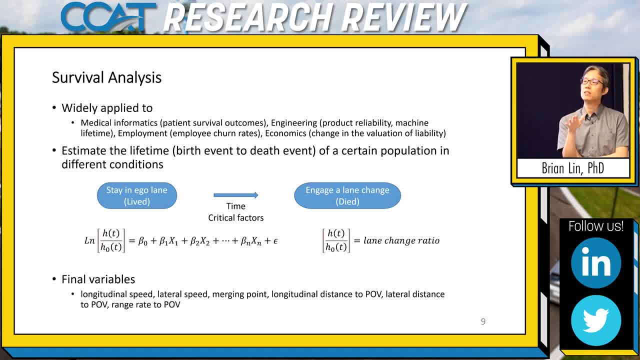 and once the time or the critical factors meet some um the requirements or the criteria, they will start to engage in lane change, which we call the dead events. so they will like, they will live, live, live, live and die. they will remain, remain, remain, remain and change lanes. so this is the 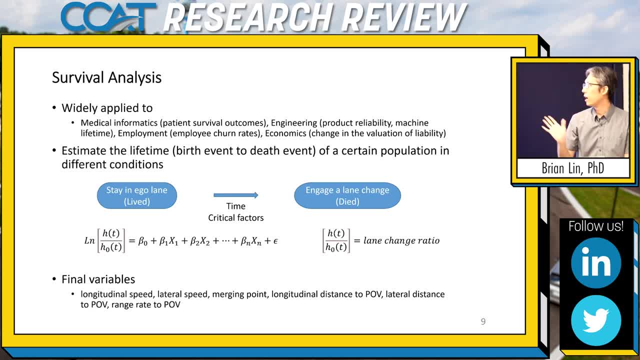 basic concept of what we, what we have used and we follow the hazard ratio functions we listed here. so we, kind of you know, change the apply that concept from the hazard to the link, from hazard ratio to the lane change ratio. so we selected: um. these are the final variables we selected from the data extracted from the 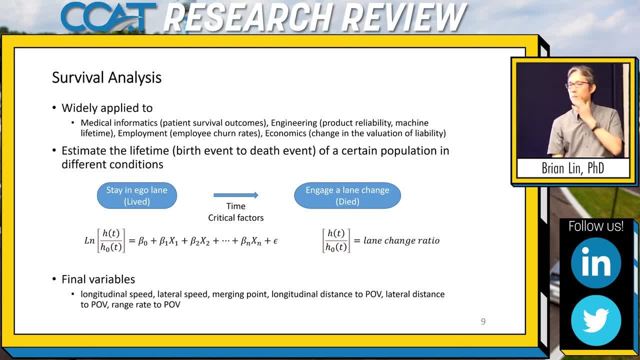 naturalistic data. so, if you um can, if you remember, in previous few slides we listed more than these variables. the reason we selected those were kind of that many of the variables we extracted were correlated to each other. for example, the longitudinal speed will be correlated to the 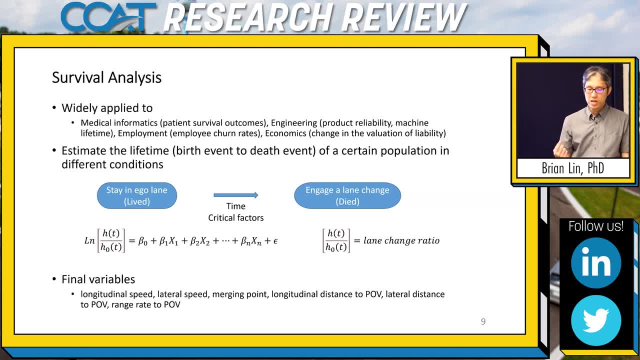 longitudinal acceleration and the lateral speed will be correlated to the lateral offset. so we tried to. we selected those variables which are more representative and also easily to extract. it to extract from the database and no further processing needed. so that's in. in the end we selected six variables. three of those are, two of those are about the ego. 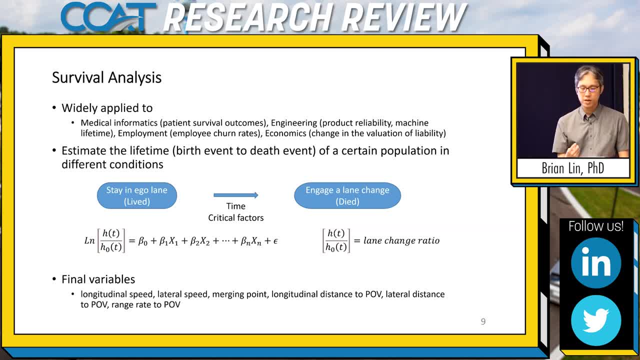 vehicles dynamic. one is about the emerging point where the lane change occurred in the weaving section, and three of those are about the heut in the inward 吧. brighter, uh, die. 1 0 0 0 0. 1 0 0 0. 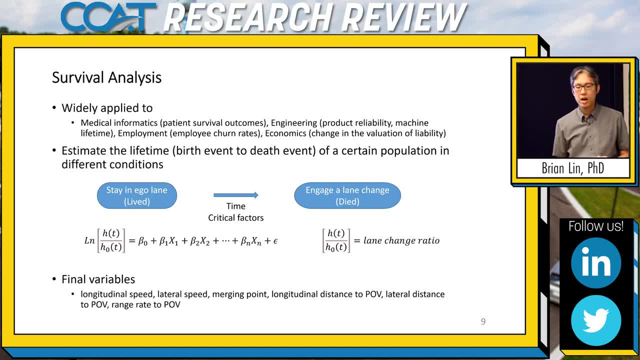 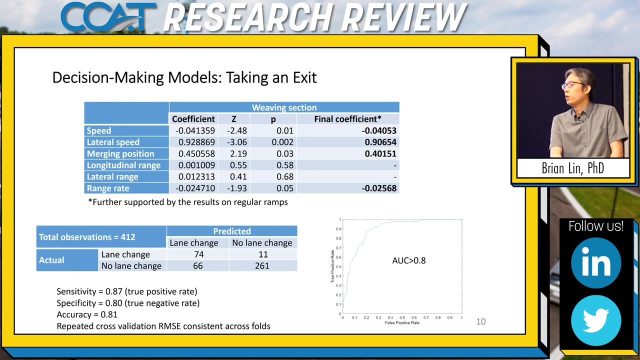 0, a classification model without using the, you know, typical logistic regression or machine learning, but we applied the survival analysis to classify the lane change or non-lane change events. so here's the first model we created, when the driver, you know, for the scenarios of taking an 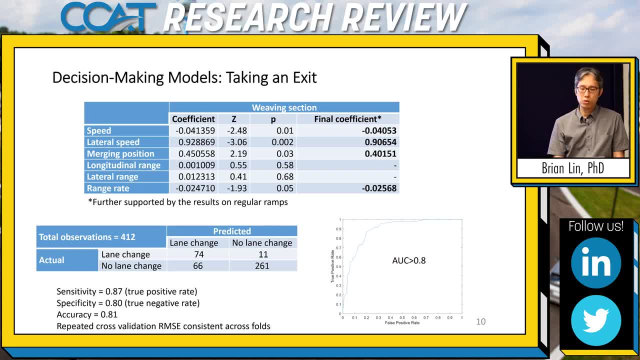 exit. so among those six variables, with the Cox regression we ran for the survival analysis. we come up with the coefficients and the significance of each variables and then we further select those as the significant ones. so we selected four out of the six and we have we come up with the final coefficients, which are the beta, as we share in the 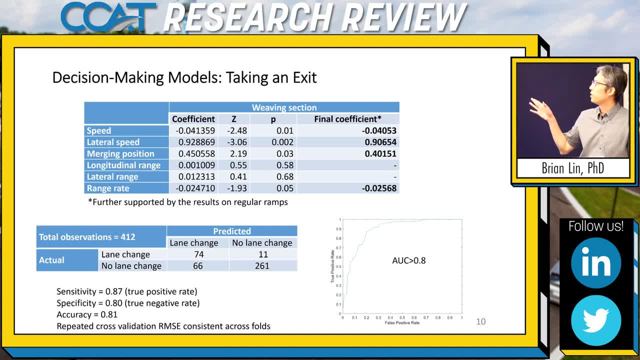 hazard function. so we use that coefficient can help us to generate the of the lane change ratio numbers and we use such numbers compared to the threshold we created from the classification models. then it help us to understand to classify if the lane change is predicted well, if the actual lane change what has been predicted as a go or no go. so 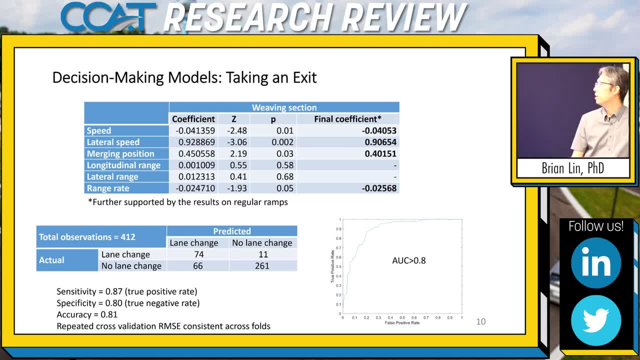 in the table at the bottom. it shows the well, totally have 412 observations to see if for the go or no go and we can classify. you know we have the sensitivity which is true positive rate. the true positive rate means you, it's actually there is a lane change and your model classified. 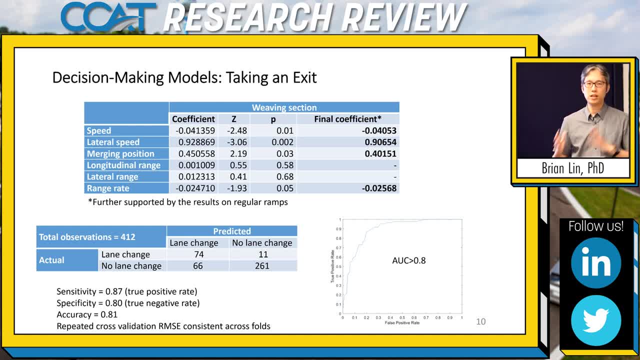 it as a true lane change, so it's just like a hit. so the sensitivity is is 0.87, which is the is good and the true negative rate that you correctly um, correctly classify those non-lane change cases when and we can identify 0.8 um of the like 80 of all the events and the accuracy 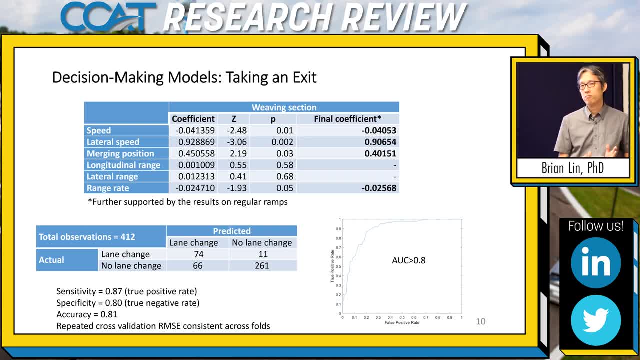 is about 0.81. so as the you know statistic models, it's kind of a convincing results. and you know the. for the roc curve shown on the bottom right, we have the aoc more than 0.8, which is with the area under the curve. so which means we can explain more than 80 of the um of the results from from this. 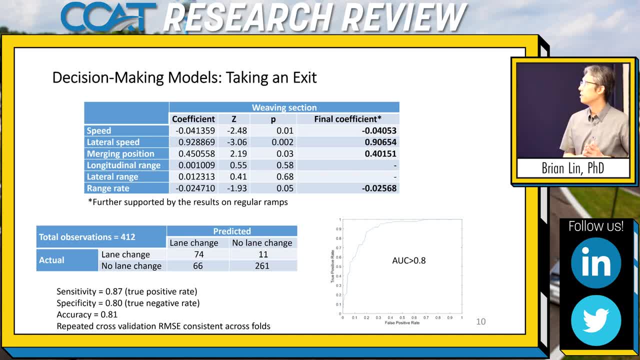 this model. so this is model for taking an exit. so again, the driver. we use the ego, vehicle speed, the ego, the lateral speed when they engage the lane change and the merging position as the ratio and the range rate to the other vehicle as the predictors to um, to predict if the driver will engage a lane change or not. 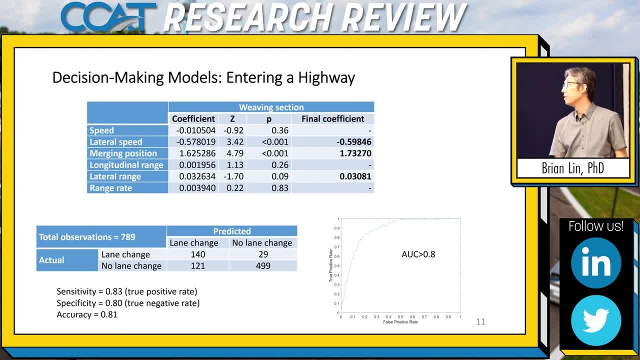 so the next page i, there is a. this is the other model, but we apply the same methods. uh, it's a when entering the highway. so it's kind of like, you know, we swap the position of the of the two vehicles, so we try to enter the highway and accelerate and merge onto the highway. 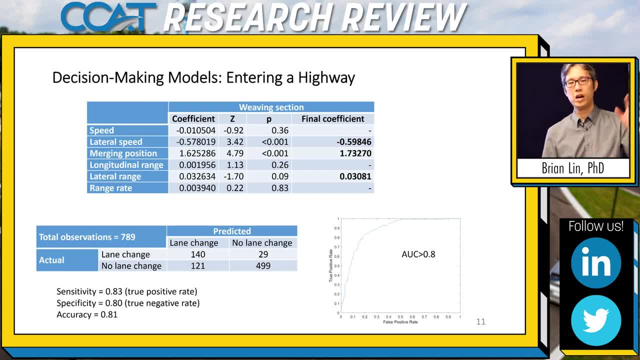 the interact with the, the road users, originally on the highway. so for the survival analysis that shows the coefficients and the significance of the of these variables, so we selected the significant, the three significant ones, significant ones out of the six. so here, notice that a speed is not a significant factor. 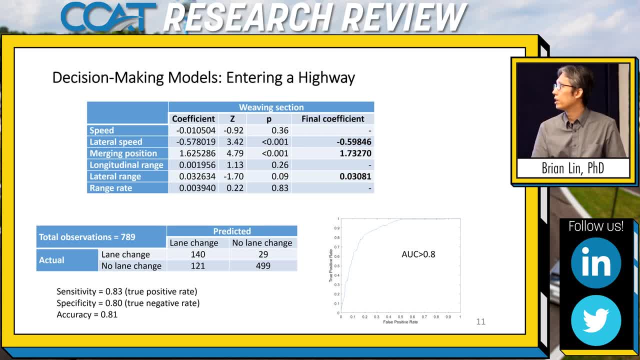 anymore, but the lateral speed, emerging position and lateral range remains and the range rate is not significant. um as well, but it was been. it's been replaced by the lateral range, but using the same method we apply to the classification models and we have total observation of 789 and that. 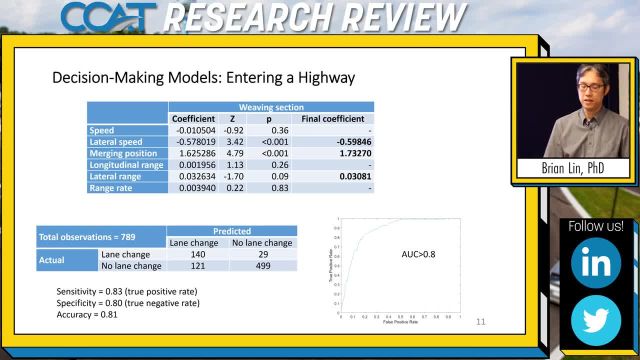 tells us: um, then apply the this should create in this confusion. matrix that shows the sensitivity and specificity of the classification and accuracy is about 8.81. so we get kind of a similar accuracy for the as compared to the, the model of taking the exit and but the prediction for the taking. 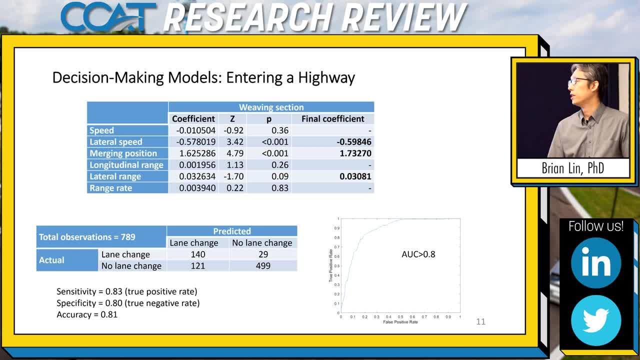 the exit has more, higher sensitivity to predict the true positive cases, but they- both models- can explain more than 80 percent of the events we extracted. so here are the models we created, um in the lab. so another jump to another topic: with the results from the lab, what we're supposed to do. there is a gap between we want to apply the result from the 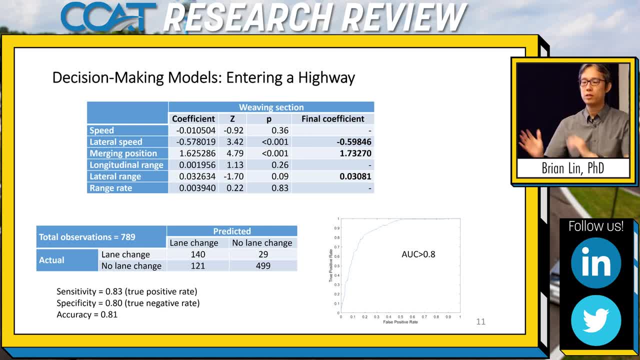 lab to either the real world or a test track. so here we ran some computer simulation to make sure it works. and even you know from the modeling parts as the computational part, we know. you know from the in the survival analysis, we know it works. but we don't know if that works, and you know when we try. 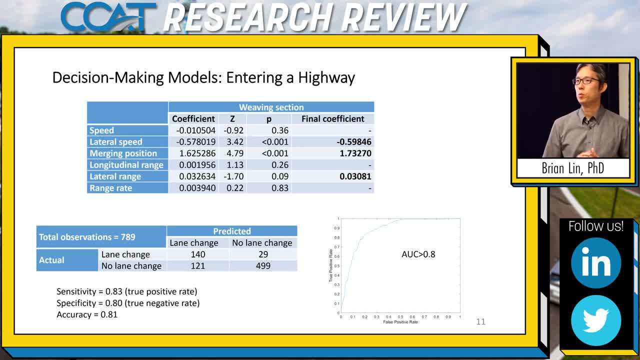 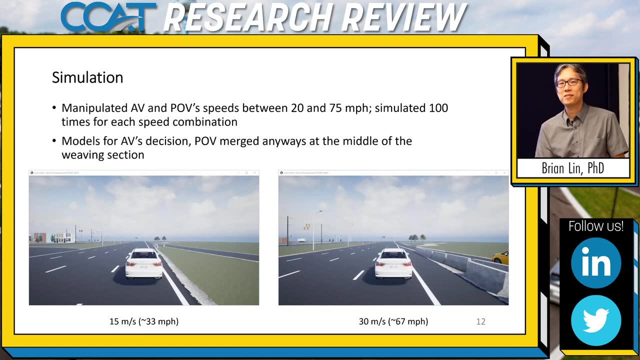 to um really apply with some vehicle dynamic parameters in a similar link and to see how we don't know if that works in the simulation. so here we ran a small um- not small, but some tests with the different combinations of the av speed and pov speed, and for each combination we sim, we simulated. 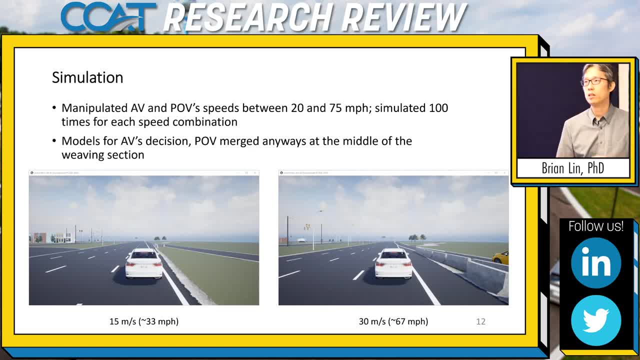 uh, 100 times and to, and then we collected the performance measures to see um, and i'll share with you what the most measures we collected afterwards. and so here i want to emphasize: what we try to model is the av decision. so we don't really, in this study, we don't really use a. 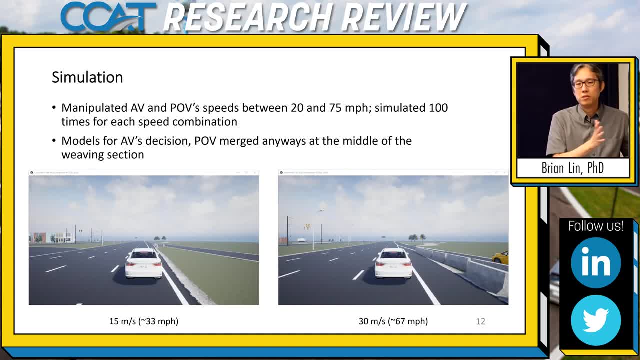 study. we don't really care that much about how what the dynamic vehicle move toward the target lane, we just want to know if the av select to select to go or no go. and to simplify the scenario, we have the um, the pov to merge at the middle of the weaving section and doesn't matter what. 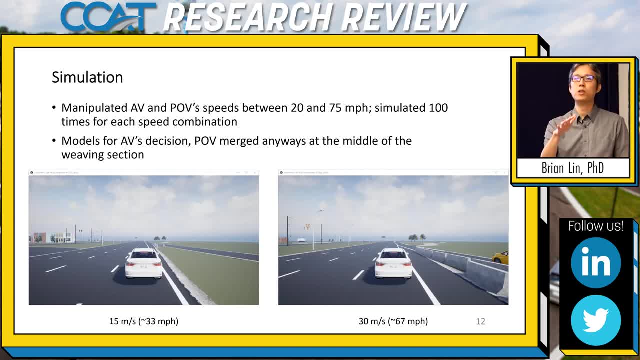 the av was doing. the pov will just merge onto the high. we'll just do what it needs to do: either onto the highway or the av will just merge onto the high. we'll just do what it needs to do, either onto the highway or the pov. we'll just do what it needs to do: either onto the highway or the highway will take the off ramp. 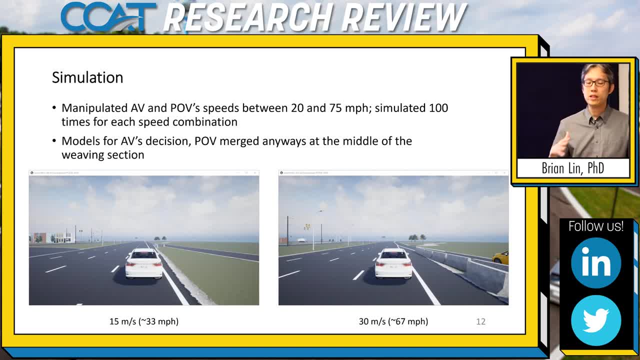 so we'd like to, with this setting, we'll like to see what the av will respond to with, based on the model we created. so here's the um, some videos i created. so the first one is the um. this simulation is, it's a 3d environment in m city for the m city facility and the av will perform with. 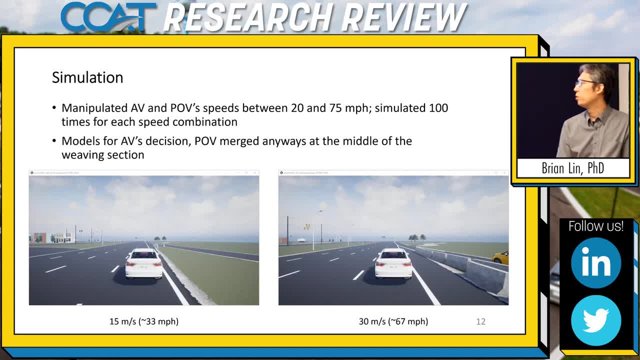 the like about 33 miles per hour, and you will. in this video you will see another vehicle merging from the ramp and the waiting section is just ahead of the white vehicle, which is the Eagle vehicle. So now let's see, in this case, both vehicles. they have the same speed. I put it that. 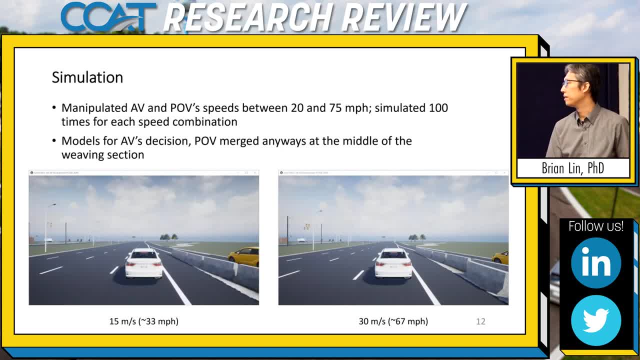 I, you know that's a default setting we have and it's very close. you know, when the the yellow vehicle try to merge of the highway and, based on our model, the vehicle is selected to to engage the lane change, I can see it's a very close distance, it's almost, you know. 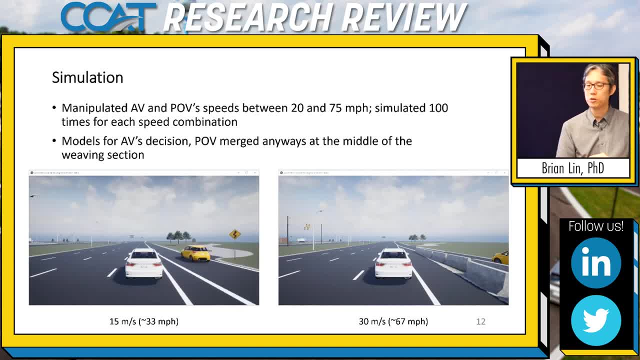 their rear and front bumpers almost touch to each other, but in our case, it's selected to make this lane change. so that's an interesting part, since this is what the human drivers will do in the real world. They, even they're- you're- driving parallel with the other vehicles, but 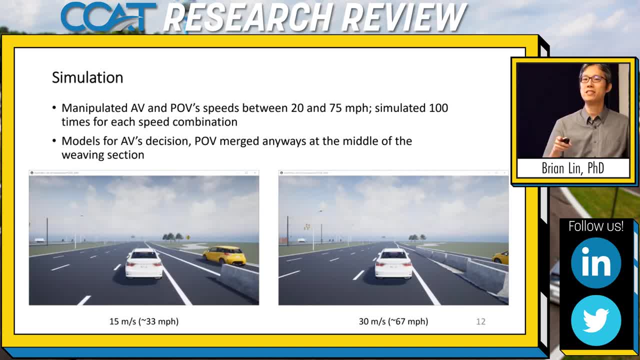 I have to get, I have to, you know, take this exit or I will take another, another 10 minutes for the other exit. so I will, I will go. even I stay very, very close to the other, the other road users. So this is, this tells us some, you know this: the white vehicle selected. 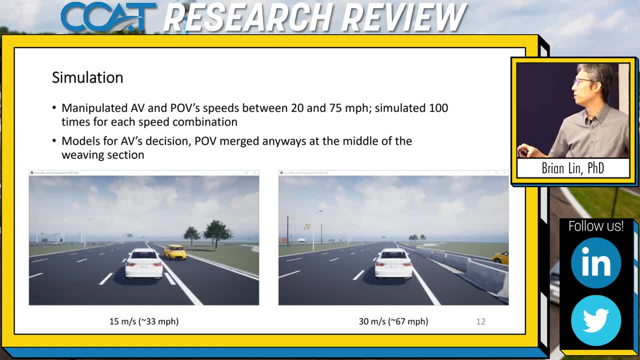 to merge onto the highway at about, let's say well, like first 40 percent of the of the merging of the waiting sections. otherwise, if they wait any longer, they may miss the, they may miss the this exit. And the other example is if we try to increase the drive of the AV speed to 30 meters per second. 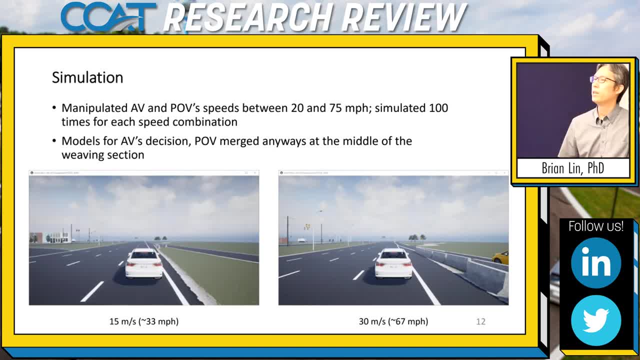 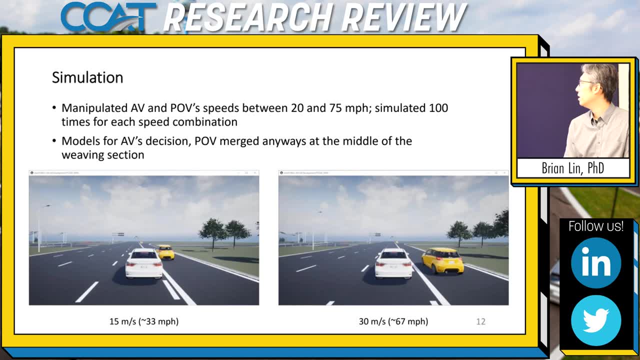 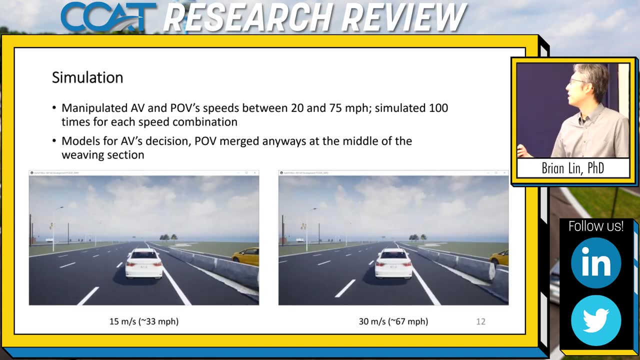 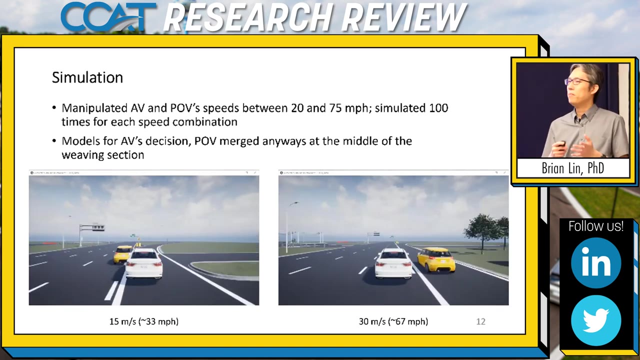 which is 67 miles per hour, and we apply the same speed to the POV. and let's see what happened to the simulation. So in this simulation you can see the ego vehicles like not to make the lane change. so this is, and again in this study we try to analyze, well, we try to model the decisions. but you may ask, 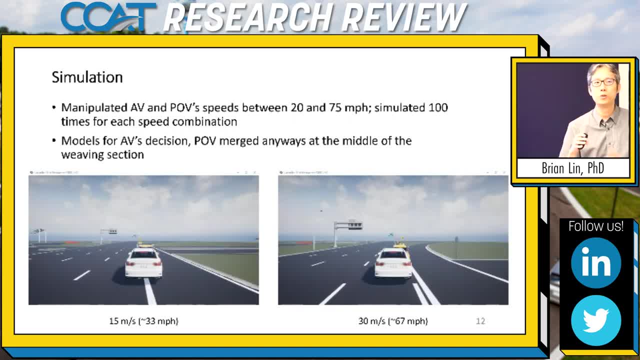 why not the legal vehicle slow down to create more, no more rooms to the- you know merging vehicle, then you can take, then you can table. so I would say that's a, that's a good point and we put that as the next phase since, well, next phase of this study, since we really like to, you know, split the. 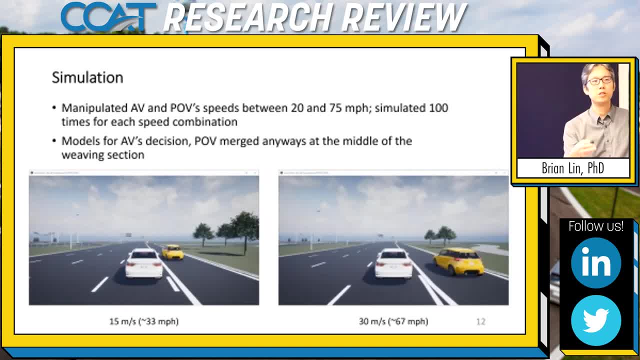 if the driver after the driver made the decisions for a no-go, what they will do next? Are they going to accommodate to different strategy of their maneuver or they will just stay on the decision they just made and miss the exit or the entrance? 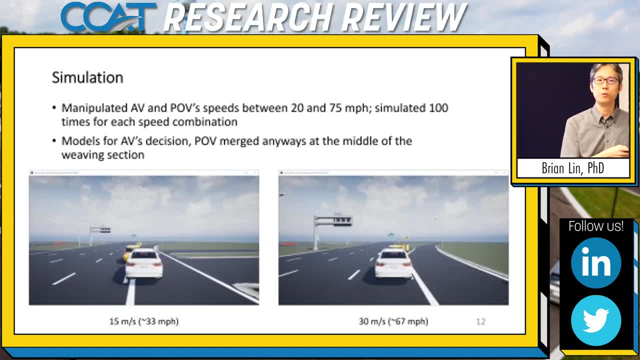 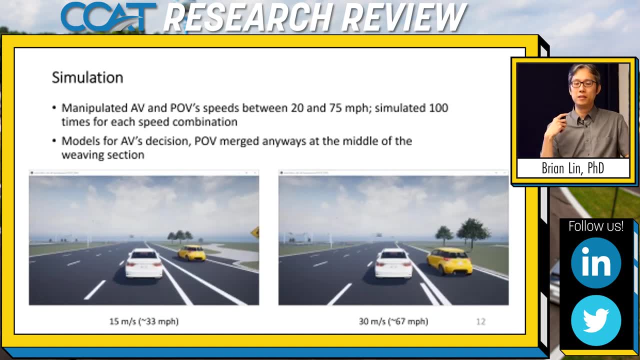 I would definitely. I'm willing to bet everyone will take the 401. But we don't know, since we again, in the naturalistic data sets we have, there's very rarely cases that a driver select not to take this. take the exit or the entrance. 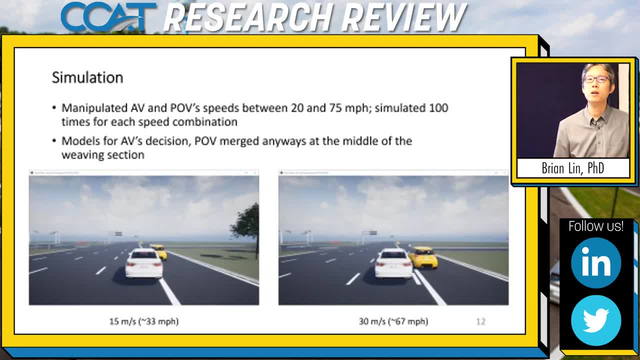 through the weaving sections. So there's kind of a limitation so far. but I'll put that in the future work if we can have for the other naturalistic data sets that can help us to, you know, to analyze after the decision-making has been made. 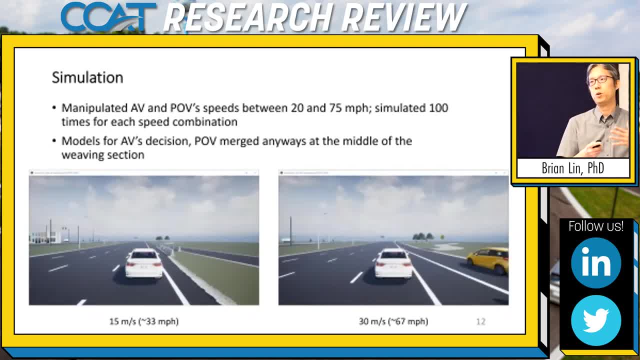 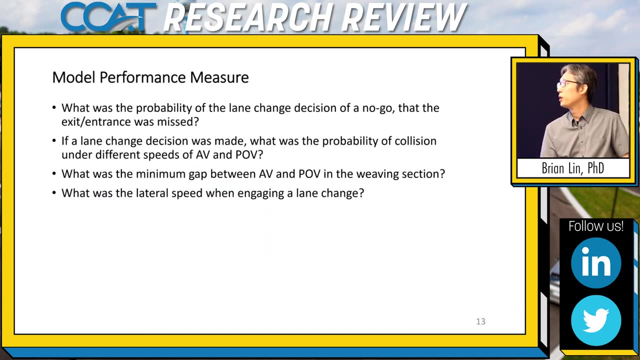 what a driver will do to you know, update the situations they just faced, and then they may change their decisions afterwards. So with these, the 3D simulations, we try to understand what the model work, how the model works. We created four performance measures. 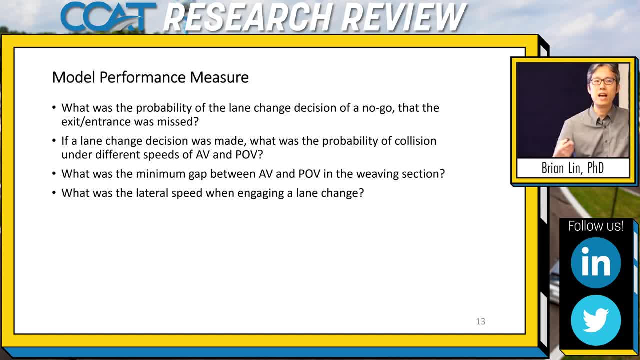 So we'd like to see, first to see if they missed any exit or entrance, and then, if they made the- if they have made a lane change decision, what was the probability of collision under different speed combinations. So again, this study will test this. 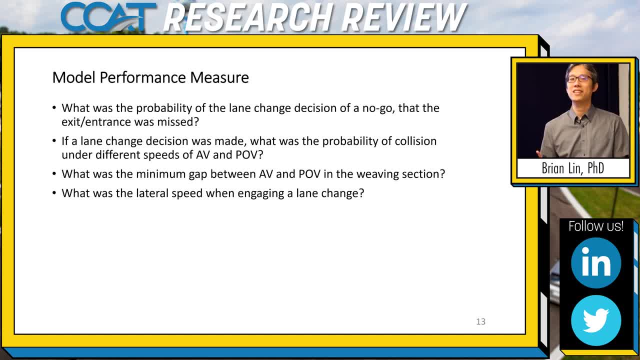 it's going to model the decision-making. It's not collision-free, So, and that's why we want to run in a computer simulation first, before we can go to the MCD or even higher speed environments. So, and then the third one: what's the minimum gap? 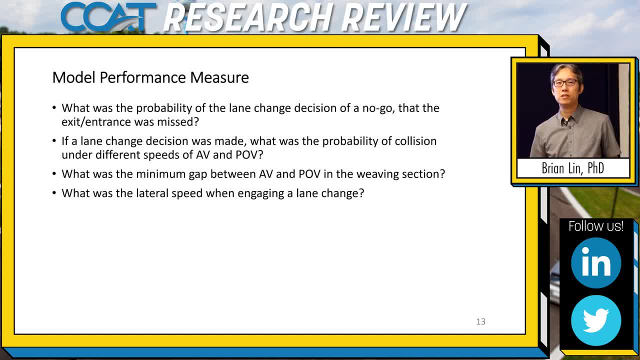 between the two vehicles in the weaving section. As I just shared with you in the simulation, you see in the weaving section and at MCD the weaving section has only 80 meters, which is very, very, very short, If you would like, if you drive on like a. 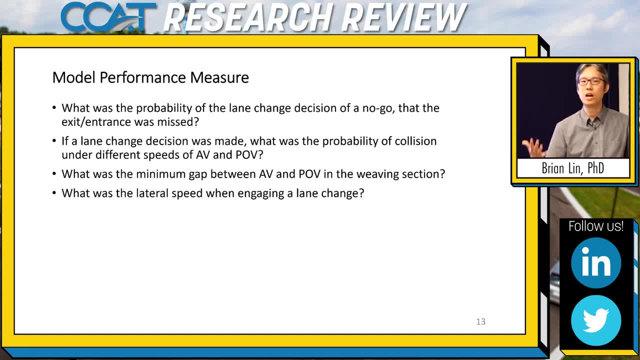 if you're simulated with a 70, 70 miles per hour speed and you will go over to that, well you will pass that in three or four seconds. So I don't think anybody can do any lane change like in three, four, four seconds. 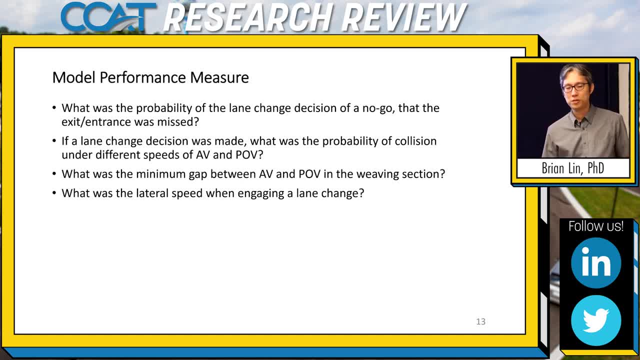 So that's kind of a lot of another limitation, So, but we simulate that in. you know, we want to do that in MCD, since it's part of the scope that we want to test in at MCD, and you know. 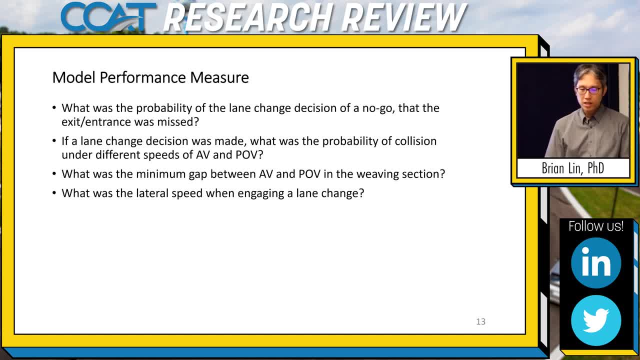 using a, using a true AV. So the last one is the lateral speed when engaging a lane change. So this one is interesting as well, Like so if you know if the driver started to merge to the exit or the end or the highway too late. 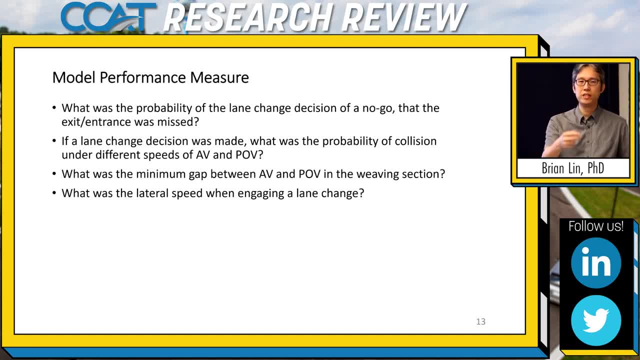 or too close to the end of the, to the end of the, the weaving section, they have to have a very. they have had a very like a huge lateral speed Before they run into the fork right. So and even we just like to know with that, 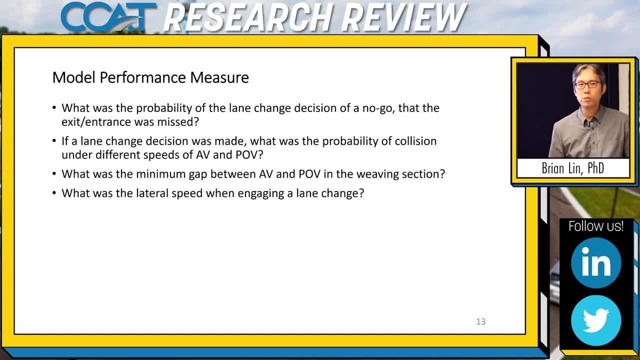 if they make the decision: okay, I want to go, I want to take this asset. what lateral speed they will like to they will like to use, depending on what speed combination they have with you know, between the AV and the. 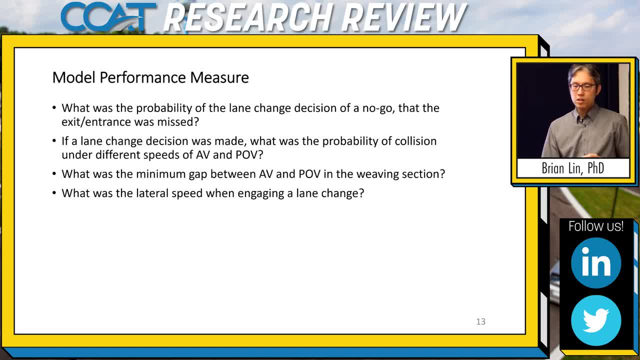 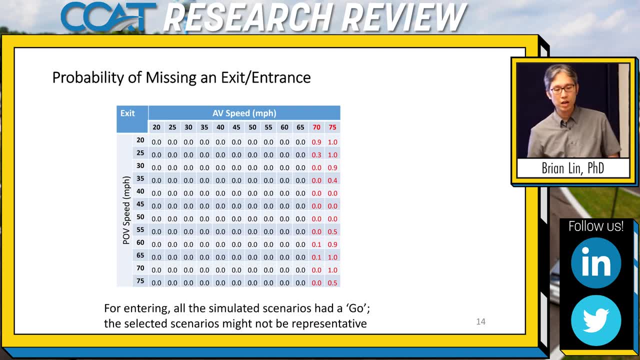 and the other road users. So the first one about a probability: okay, before they run into the fork right. So, and even we'd just like to know with that, if they make missing an exit. It might be a little bit tiny, but I don't want, I don't need you to read through. 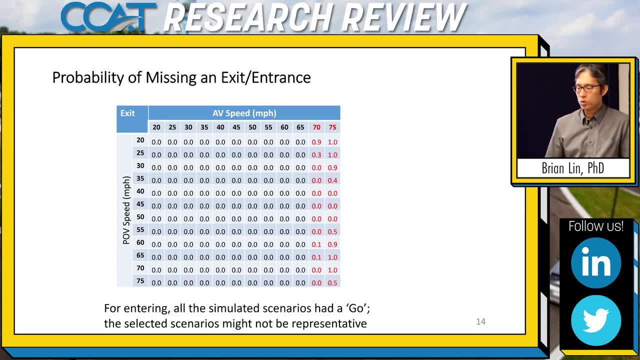 the numbers here. Just take a quick look at the red numbers So you see when the driver, when the AV speed is 70, 75 miles per hour and the POV it's about, you will see many. in many scenarios the probability of missing an exit or entrance will be very high or even close. 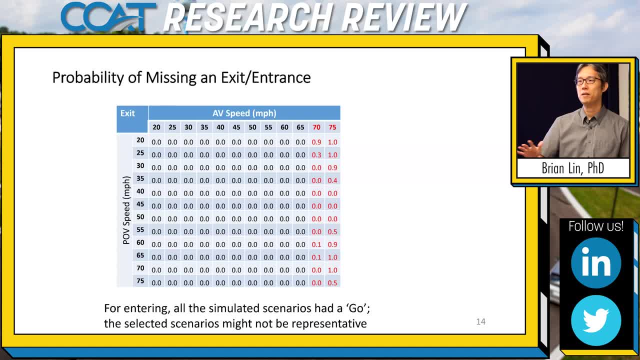 even just one. So in this case, in this settings, the driver will definitely miss the exit or entrance. But again, this is the simulation at M-City. So at a 75 miles per hour you have only three seconds, four seconds the most, to merge and do away very easily And to you know, 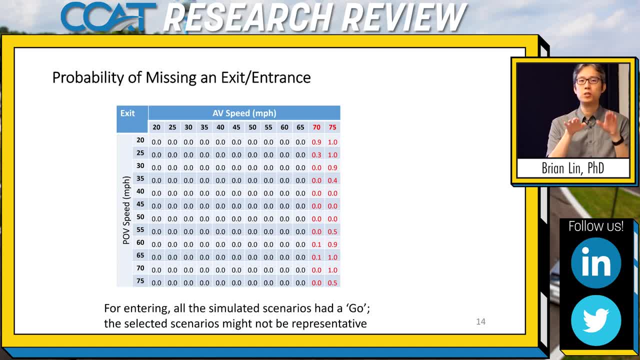 any tiny, you know, adjustment of your speed of the, any tiny adjustment of the speed of the AV and the POV will affect the results. So that's why we ran this simulation for one, like a hundred times. It can be more, but a hundred times is good enough. And then we see, you know. 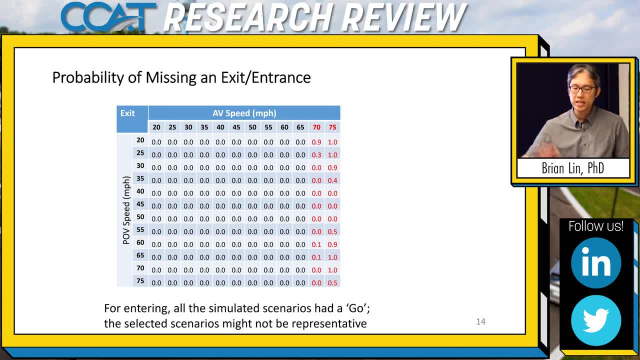 especially when the AV is, you know, 75 miles per hour. in many cases, you'll see, the driver will just miss the exit and entrance. Well, sorry, the, the um, the, the exit. The interesting thing is, from the model for the entering, um, all the simulated 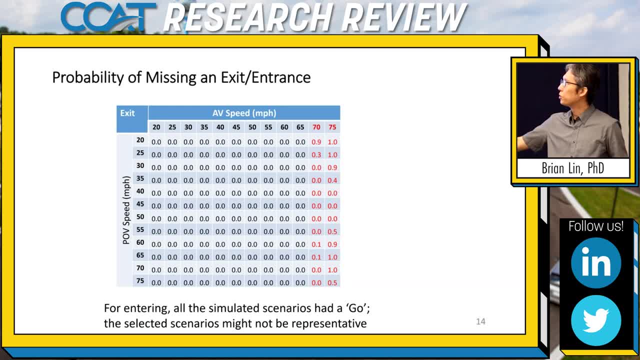 scenario had a go So different to the? um, the exit scenarios here. um, we found that's interesting. that which means any, the driver will merge, will, will get onto the highway anyways. So, um, it's not they will miss, they will not miss any entrance, They'll just get on the highway. 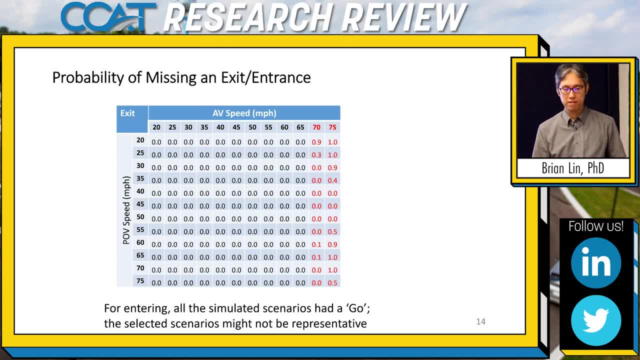 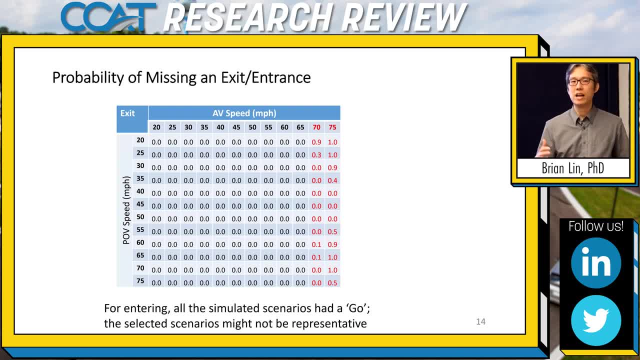 data um saying the driver was actually expecting the. you know the response of the other, the, of the other road users on the highway, And if you remember the significant factors we um created from the survival analysis for the um for entering the highway scenario, 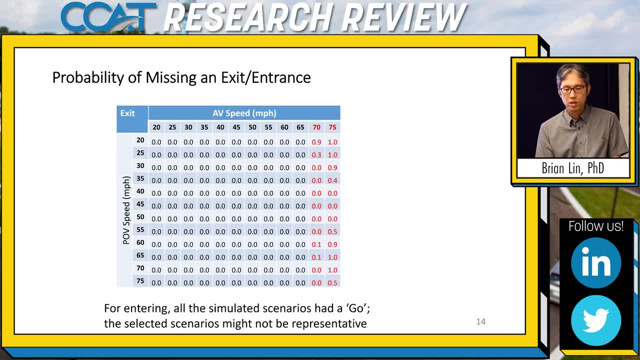 there, there is no longitudinal variables. We found the lateral speed, We found the lateral position, well, lateral distance to the POV and the position of the merging point. So there is no longitudinal, um significant longitudinal variables, which means which? well, I think that that that 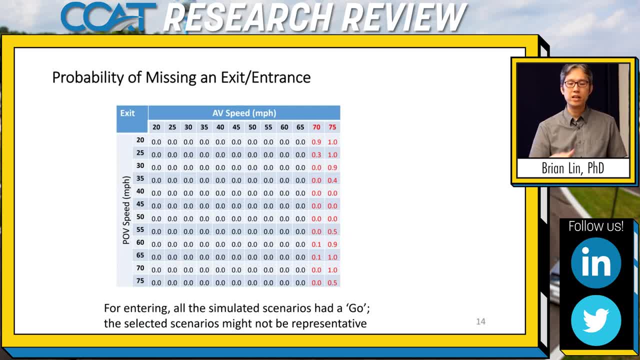 implied. the driver tried to uh, take the entrance onto the highway. expect the, you know some lateral plates. So all my 때는 control from the um, the the road users originally on the highway, either to get the way to them by slowing. 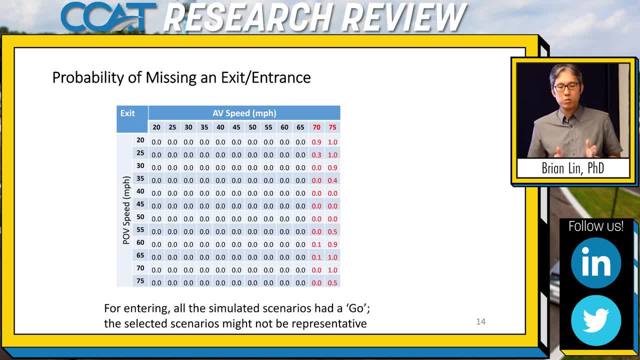 down or passing them quickly, But they will, since we will run all the way. we'll run all this, the weaving section, very quickly, very soon, especially with the high speed of the AV. So the driver will drugs know merge anyways. so this is the first performance measure and the second one: you just a lot. 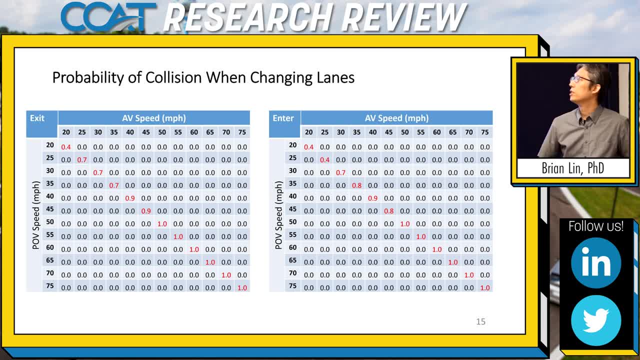 of numbers here are zero, which means no collision, but it's if you see the numbers on the diagonal and when the faster the driver, the faster the av drove, the higher probability the collision movie. so that makes sense since um. so, for example, if we just drive at 20 miles per hour with the 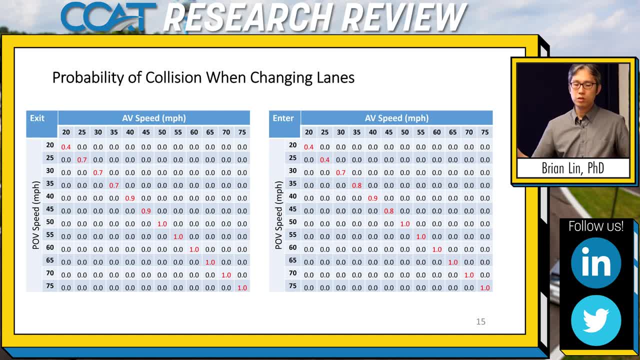 speed of the, the pov, the collision probability has only like 0.4, so which means you have more room to adjust your decision. you have one more room to you know, or more room or more time to make to before you make the final decision, So that lower the probability of collisions. 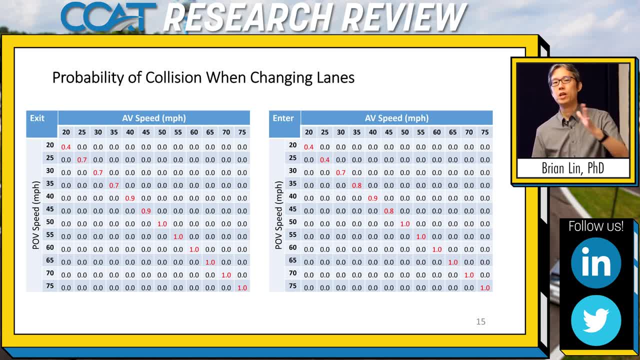 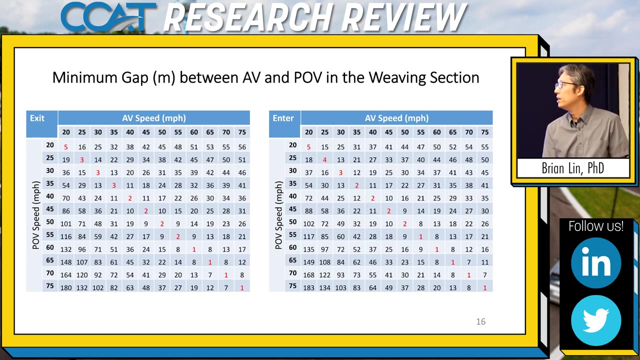 And in the AV. when you increase the AV, driving faster and faster, you have only three, four, five seconds and there is no way you can make the lane change without the collision. Otherwise stay on where you are and select no go. So the next slides about the minimum gap. 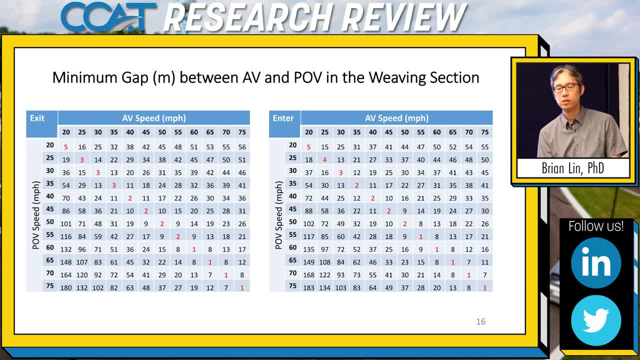 is kind of a something related to the previous one as the collision rate, the probability of the collision. So if you see on the diagonal this, the minimum gap are very short: two, three sec, two or three meters, Some of those even just one. 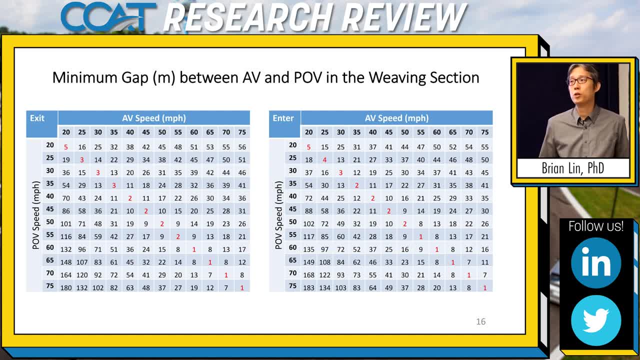 So it's kind of a you know, and, as the computer says, this is just a simulation and I don't know what's going to happen in the real world. So, which means, if we for this with this model, if the drivers select, you know. 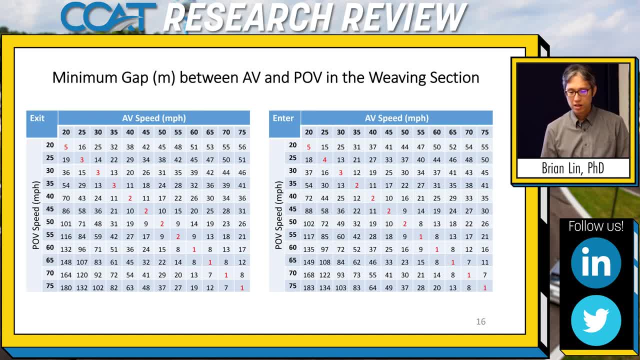 stay with the same speed as the POV. there's a very, there's a, you know, very high probability. they will have some collision into each other and they will have the minimum gap will be very, very short. So even some of those you see like 10 meters, 11 meters, 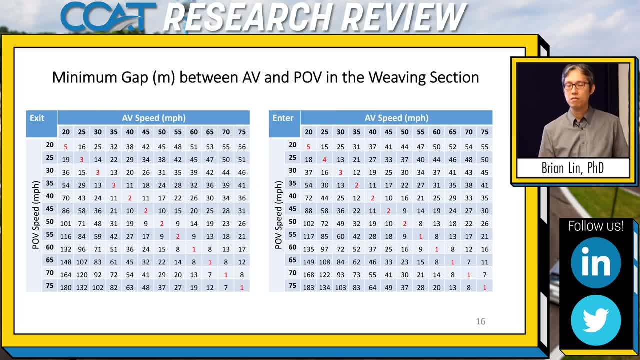 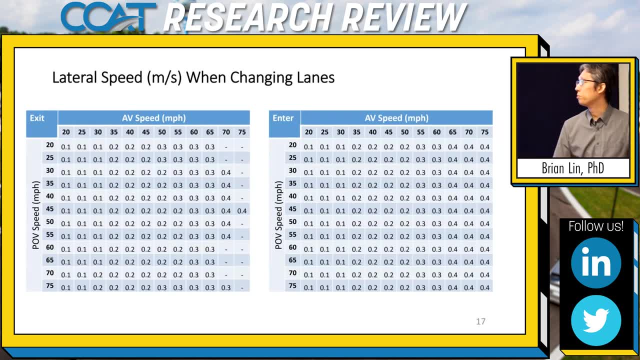 but at high speed it's very small And for we also estimate the lateral speed when they change lanes. So it met our expectation that the faster the AV, the faster the AV has the lateral speed it needs to apply when they change lanes. 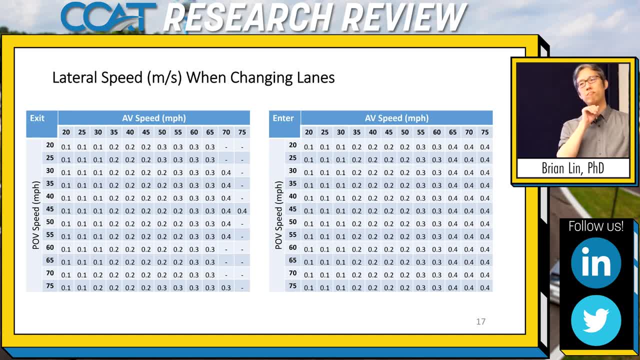 So they try to engage the lane change, Otherwise they may, you know, since they have shorter time, so they need to move faster laterally in order not to run into the fork of the weaving section. So about the summary of this, the simulation. 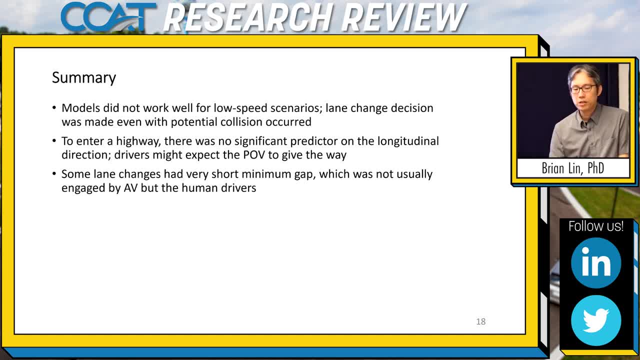 we found that you know, the model actually will did not work that well in the low speed scenarios, Since, well, you find, you see, in our, in those on the matrix. I just share with you the low speed scenarios. 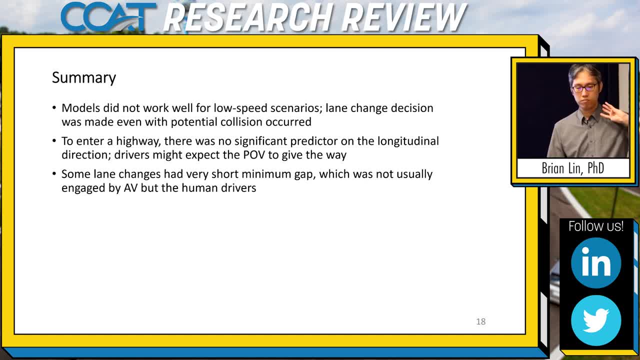 many of those. okay, there is no collision and they will just go anyway, but you will see some. well sorry, you'll have a high probability of making a decision of a go, but you also have some probability to have the collision. 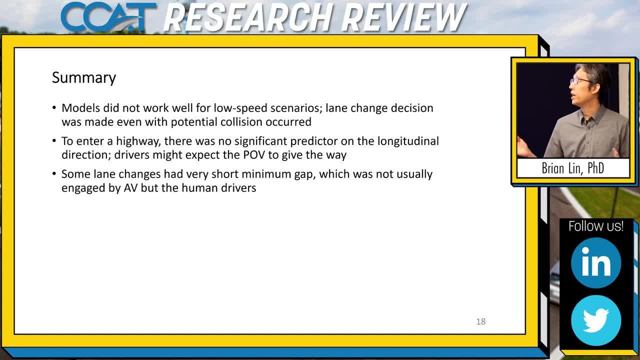 with the POV And again the lane change decision was made, even with a potential collision occurred. So the reason is, when we try to model the well first, it might not make that much sense if you keep them at a lower speed on the highway. 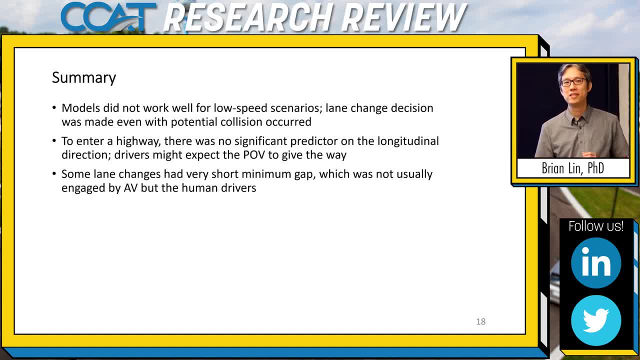 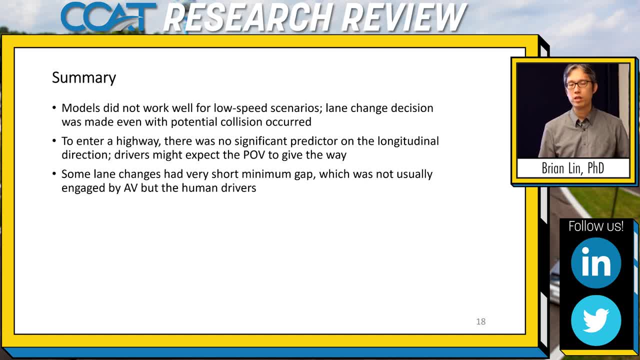 entering events. so, in other words, when reaching you know, the, when reaching the starting points of a weaving section, most of the driver had already speed up from you know and stay at the end- not exactly the same as a speed limit on the highway, but close to. so we have more. 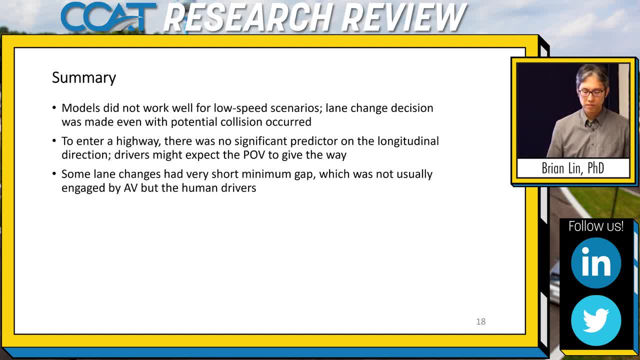 cases on the moderate speed or higher speed ones, and, as i just mentioned, to enter a highway, we found no. um, we found no. well, in other words, all the events, all the prediction of the events has a go. so the driver would, will make a lane change under any kinds of a speed. 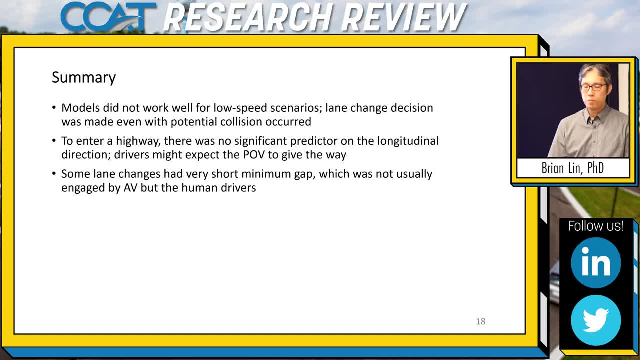 simulation? well, any kind of speed combinations. so our explanation is that there was no significant predictors on the longitudinal direction and the driver might expect the pov to give the way, so they would just select your merge and let the other road users to avoid the collision. but in this simulation the pov just follow the preset routes, so there is no collision. 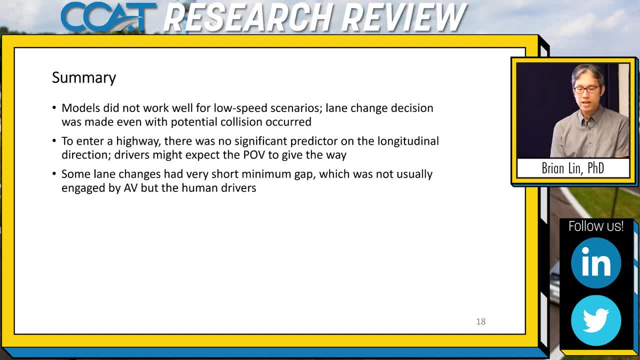 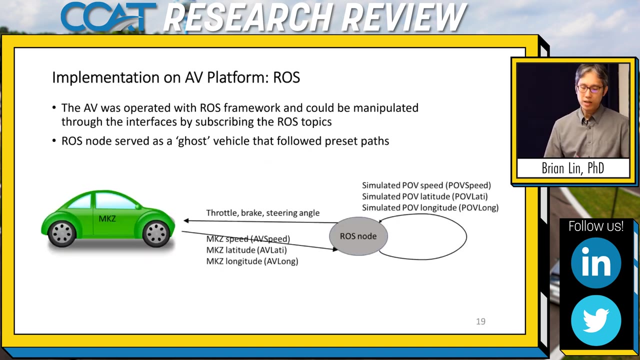 can be avoided by the pov itself and some lane change had a very short minimum gap and you know, which is not usually engaged by an av but very possible. you see, from the many of the human drivers on the road you see it every day. so the last part of that, we try to um the av. we try to implement these models into av platform. 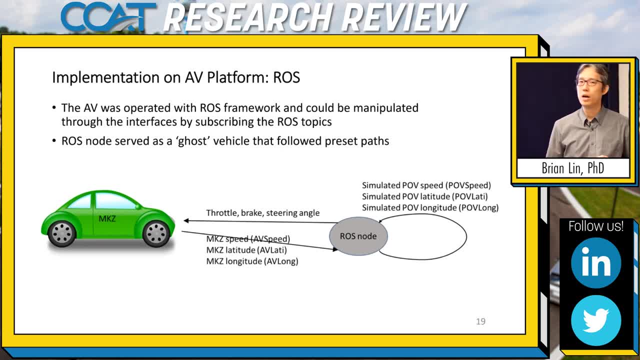 so i will um, i don't need to focus more about too much about the technical parts, but, in short, we tried to. we create the like, a rosno to control, to create um, to you know, serve as the ghost vehicle. so it's, since it's not a collision free model yet, so we cannot, uh, or we were not allowed. 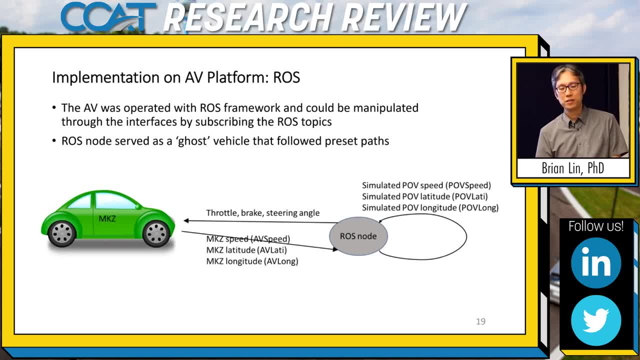 to before we, before the- you know, complete of this project. we are not allowed to run the study with two vehicles, so we can only do that with one av. but i can create the ghost vehicle to interact with the av to see how that models works. so that goes: vehicle will send um, we'll send a. 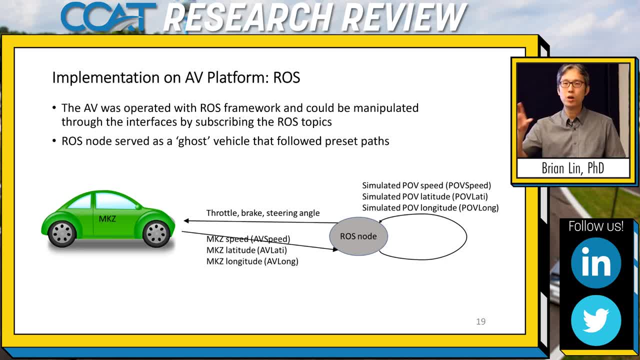 command. well, it has to calculate that it runs the model in this scope. this goes vehicle. and then we'll send a command- the throttle and brake steering angle command- to the av to ask the av to do something, and the av will send its speed and position back to the ghost vehicle. so the ghost. 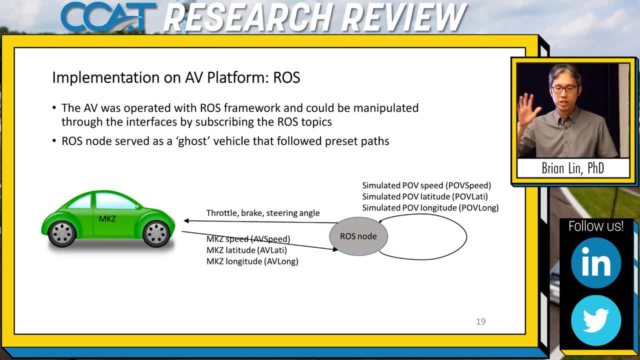 vehicle knows where the av is and you know the model can calculate and send back to the av. for now you need to make some steering because, because this is the command that want the av to make the lane change. so that's a simple concept of that. so here's the demonstration: um, like we create. 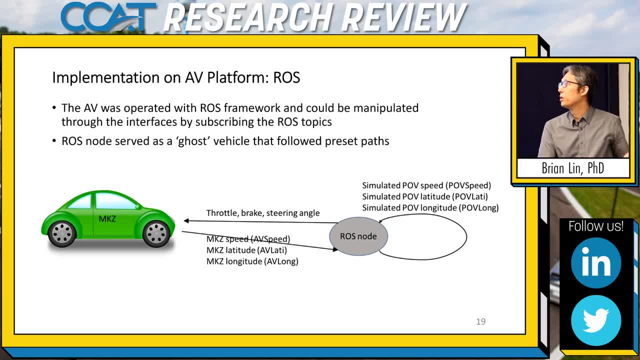 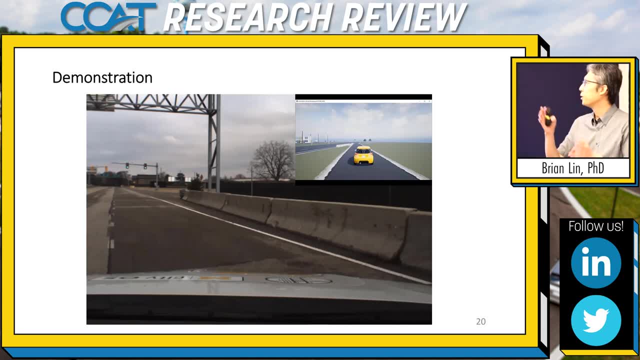 the. we use this platform, we create a video. that's kind of a concept of the augmented reality, but it's uh, just easier for you to understand. there is no, and in the, in the big um, in the big screen, there is only davy on the field. no other vehicles. but we um, we implement the well, we import. 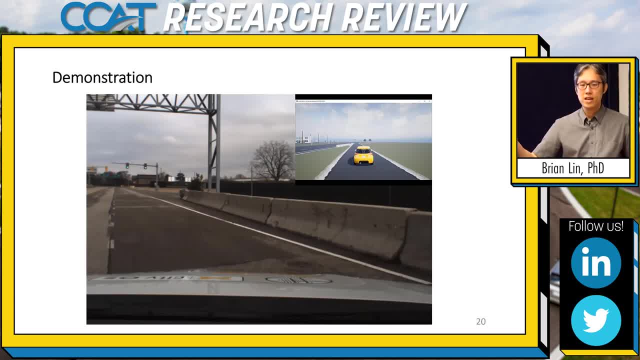 the model from the ross nodes to the simulink, and we synchronize these two videos. so we just pretend there's a um, a pov, a yellow colored pov try to merge onto the highway and the um- the av itself is going to. it stay now. it stays on the highways, tries to merge to the exit. 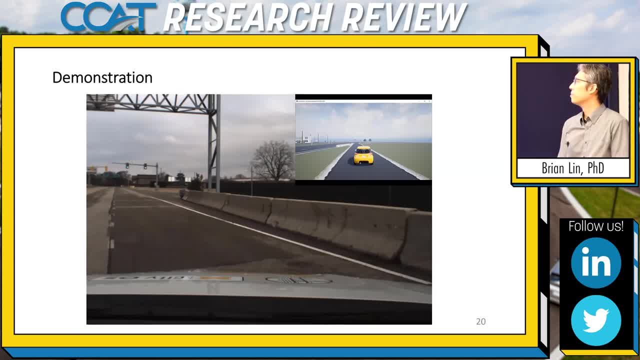 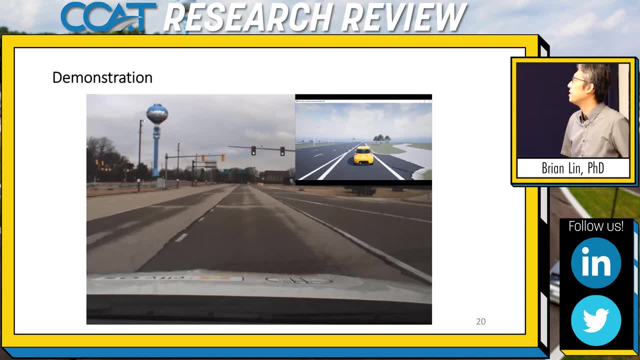 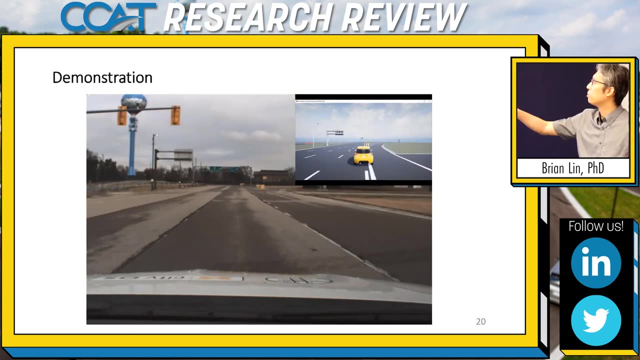 so this is um after the synchronization. this is how the model works and it's not a very um urgent event. so we see now the, the pov is probably at the center, at the middle of the weaving section, now across the board the light boundary and maybe select to to move. 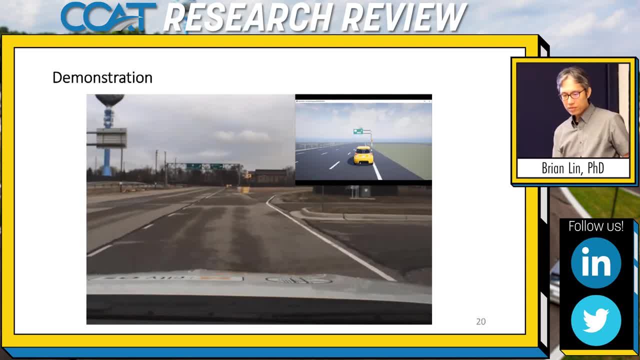 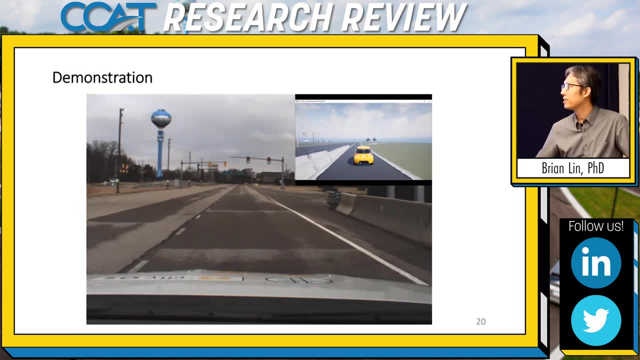 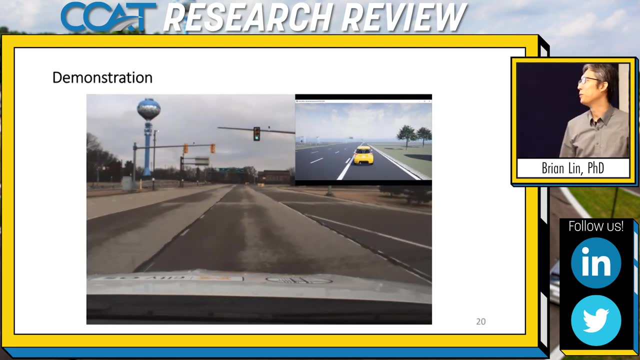 so again, um, we here, we try to control the lane change decisions. so you can see, like you know, after the latest main chain decision has been made, that baby has the like, a little bit of a like, a sharp turn to the right. so it's not perfect yet, but right now our goal is to try to to make 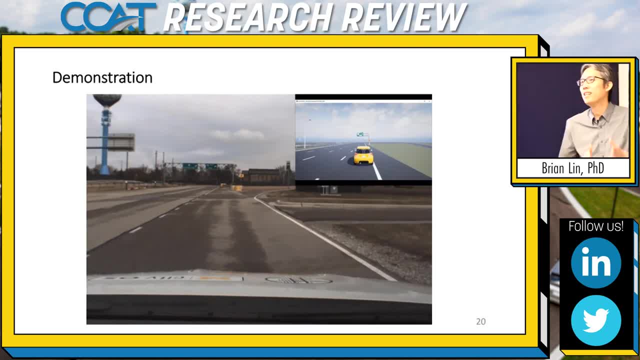 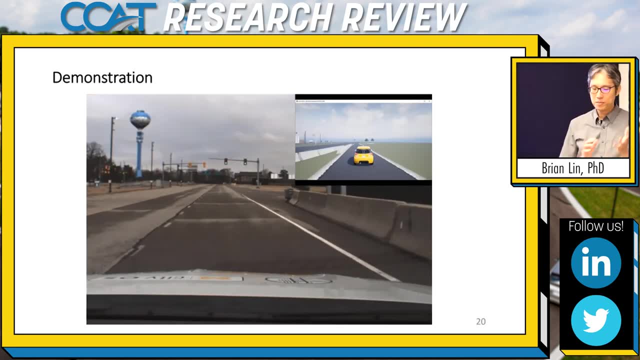 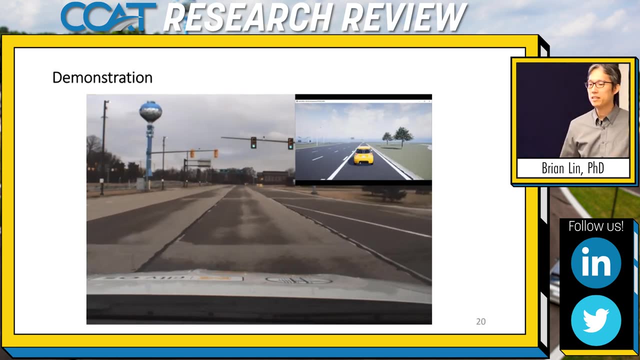 this. you see that's shuttered to the right back, so it's not the you know, smoothly lane changes to the um, to the exit. but i think it's our goal is to, you know, make sure the decision decision model works. and so, again, some of the the model works in some of the situations, but not all of these. 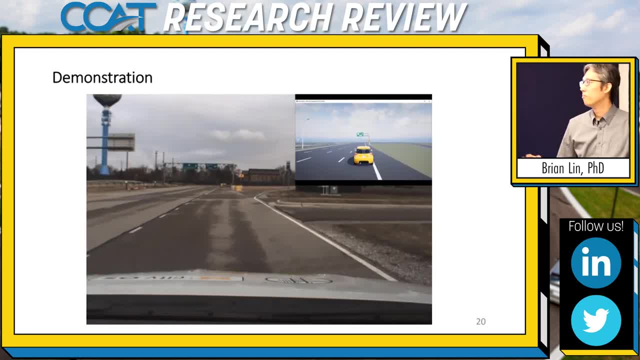 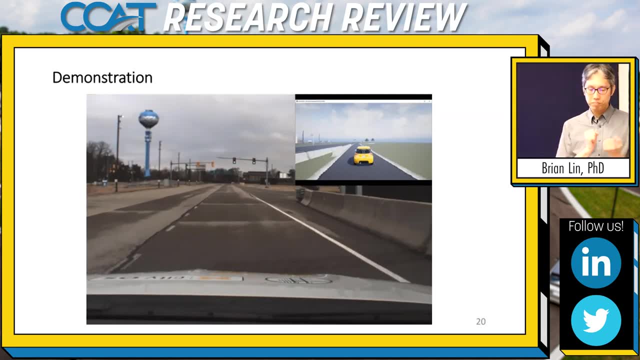 are good. so i'm going to go through how you do this, but first i'm going to break down the aerial. yeah, so one of the reasons is that the, the, the, the�� is the, the one. the theve works for the. i don't know the triangle and how it works, but the theve works. it takes a lot of. 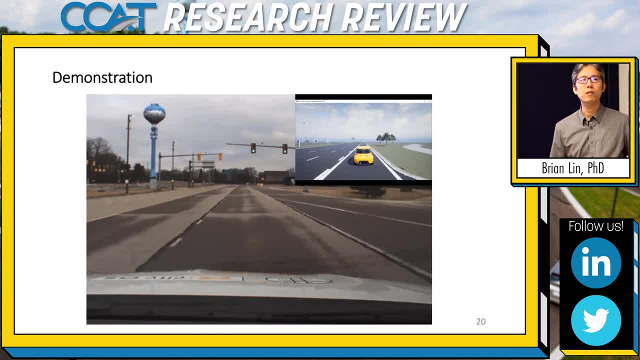 time to figure out how to do it. so we're a very complex group, like we're really working on parallel lines, so we make a lot of work around these lines. you know the ones that we're always introduced to, that we're the final ones for which we're going to look at them in detail. 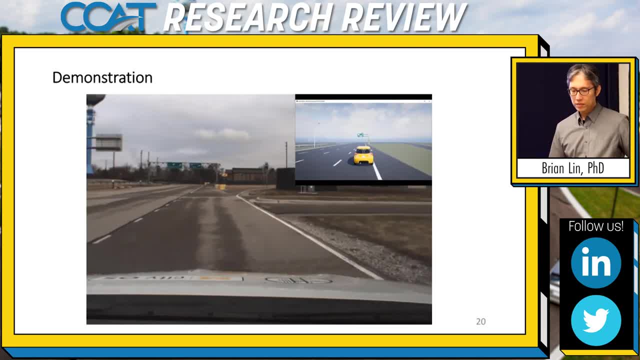 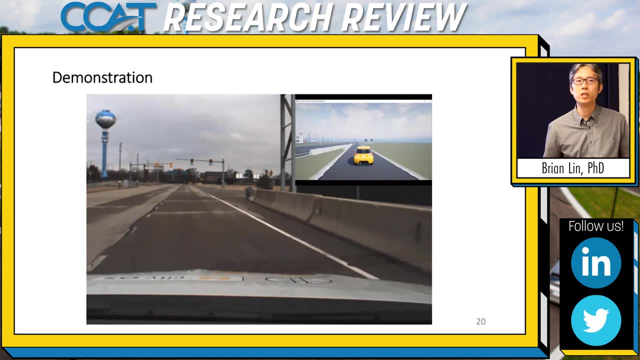 and so this is like what i set up before: to try to figure out how to do this. so, as you can see, if i'm just doing a little bit of this, so that's how it works, some evidence that we can successfully apply or implement our computational 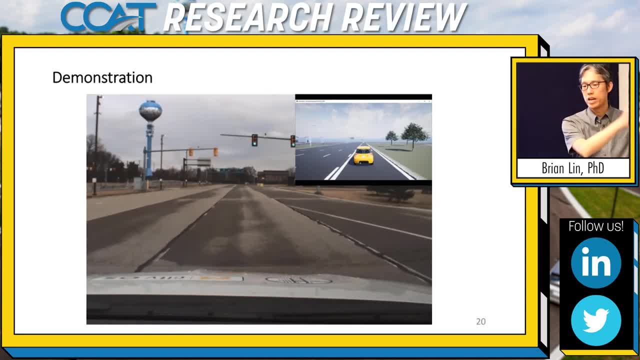 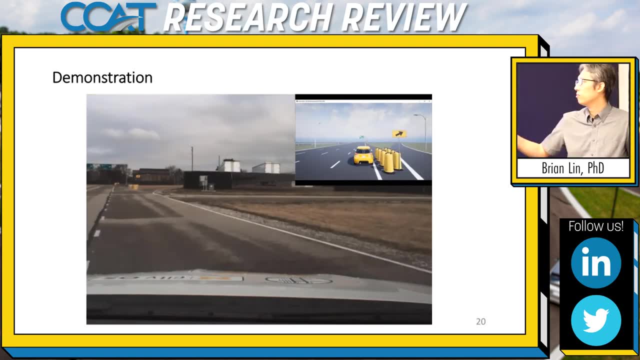 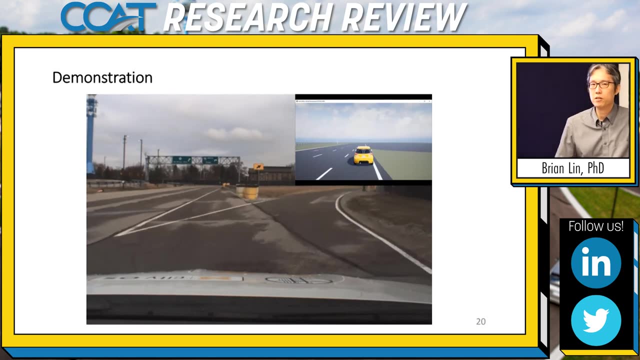 models and we cross the gap between from the data to the real world that we can really apply our models into a true AV. So now it's just like a lane change models, but we can do that for all the other decision makings and even the 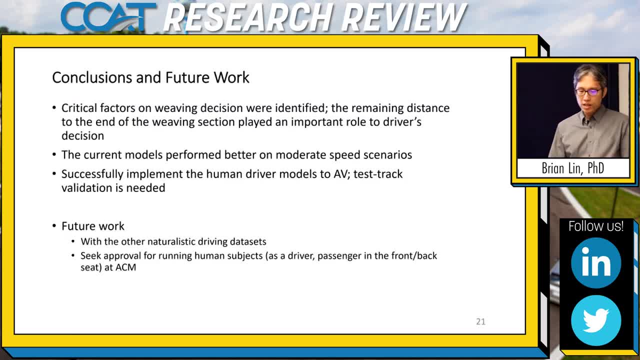 maneuvered models we have in the future. So by the conclusion, you know, in this study we have identified the critical factors on the weaving decisions and, based on the naturalistic data and we know, the remaining distance to the end of the weaving section played a very important role comparing to the other factors. So 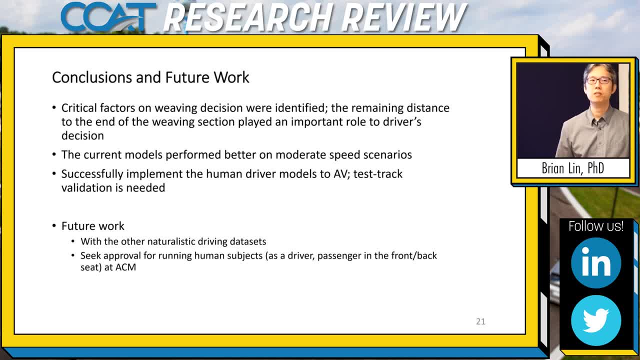 in perform better. the current model performed better on the moderate speed scenario, Since we don't have much data for the low speed scenarios and the simulation we ran at M-City is not a like a appropriate environment for high speed scenarios. So that's but for. 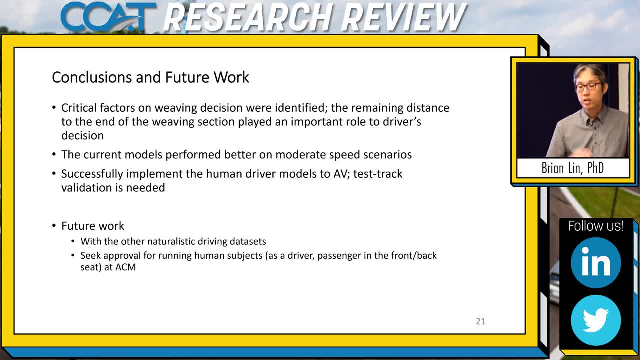 the moderate speed scenarios it works well and we can successfully implement the human driver models to an AV on the test track. But the next thing we need to do is to validate the results. So I said sherry in the video is just a demonstration, So we did not collect the data on that. We just want to see if that works. 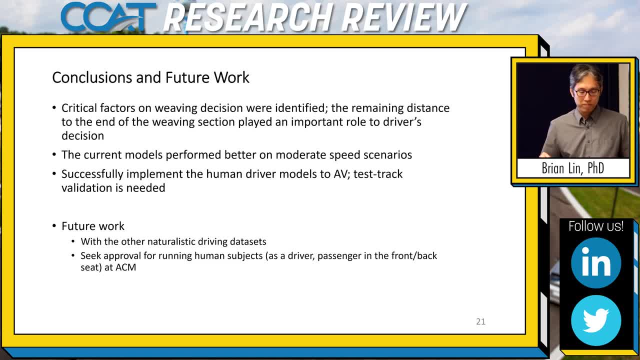 So in the future we'd like to use other naturalistic driving data data sets and you know, with a longer range, wider range of the speed profiles. And then we also like to see, if we are very keen to see if this kind of study can be applied. 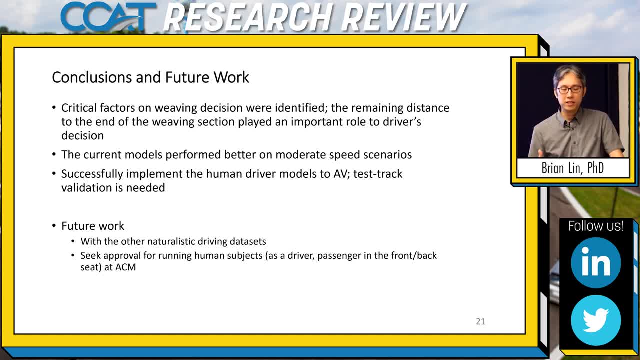 We also like to see if we are very keen to see if this kind of study can be applied. So the next thing we want to do is to validate the results. So that's what we did on the M-City test. Next thing we want to do is to validate the results, And then we want to see if it's going well. 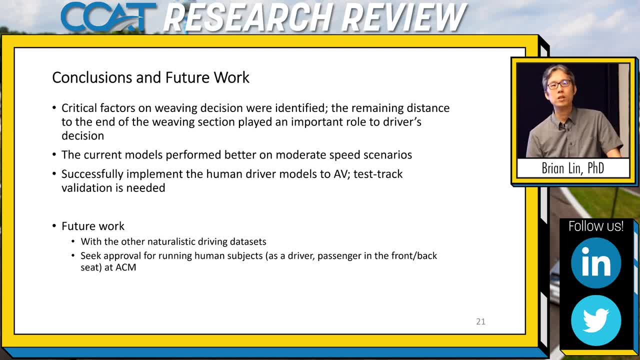 keen to see if this kind of study can be approved for human subjects running. So one of the human subjects as the driver, as a passenger in the front or back seat, and ACM will be the more ideal environment for us to apply the high speed driving environments. 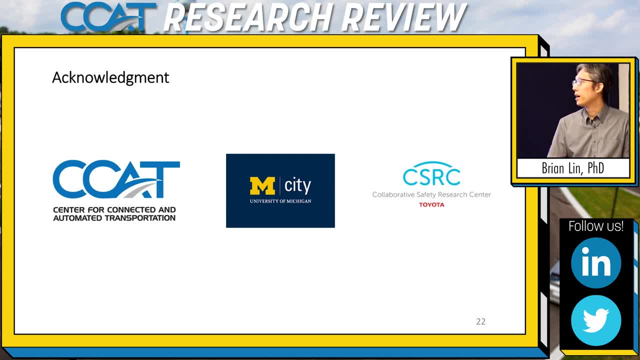 So thank you, and I also like to appreciate the funding support from CCATS, the support from MCITI for the test facility and the automated vehicle, and Toyota CSRC just served as the champion of this project, Thank you. Thank you, Brian, We have some time for questions. 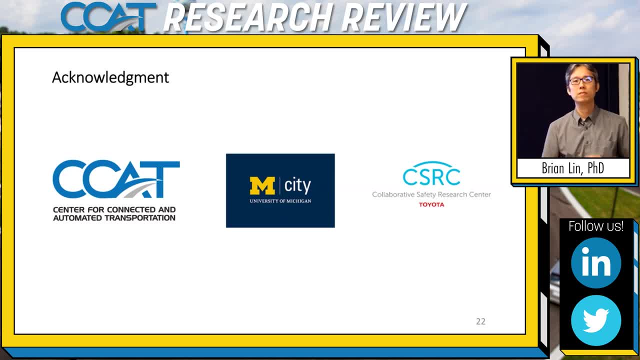 So the first one is: was this analysis related to time or fraction of time available? So well, the question is: do I need to repeat it? Yeah, over here, Okay. So the question is: is the analysis associated with the time or the time fraction? 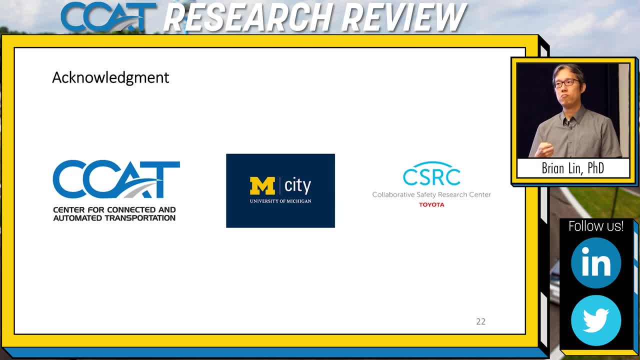 So, yes, So that's why we selected the survival analysis than the machine learning analysis. The time plays an important role and also the time was related to the merging point. Okay, In other words, the longer you stay in the weaving area before you make the lane change. 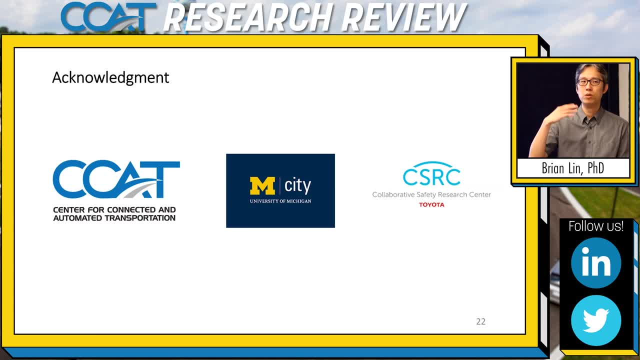 the shorter distance you will have before you run, before you approach the end of the weaving section. So the data point we collected was actually from for a five second window from the started, from the: the merge of the well, sorry, the merge of the well, the merge of the well. 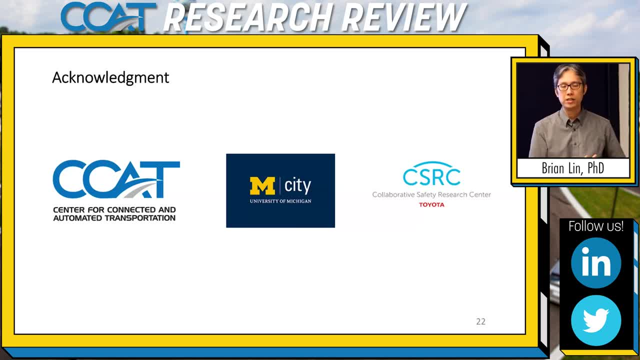 well, sorry, from the lane change and trace back for five seconds. So we'd like to see during that five seconds. So we have no go for five for four seconds and a go for at the last second. So that helped us to create the classification models. 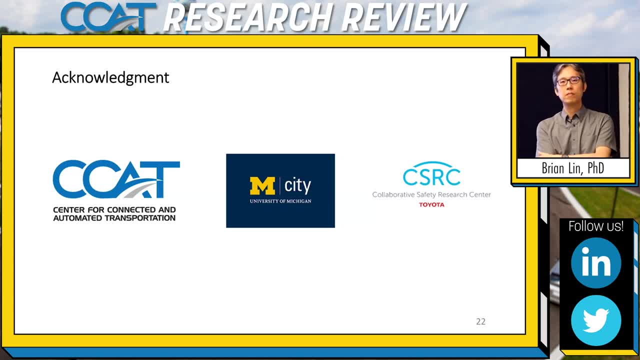 All right. So from a time perspective, the analysis was normalized to like available time. That was just a follow up. Yeah, So so the the question is: is time has been normalized to the? has the available time has been normalized? So basically, we try to. you know, we, we try, we we make. 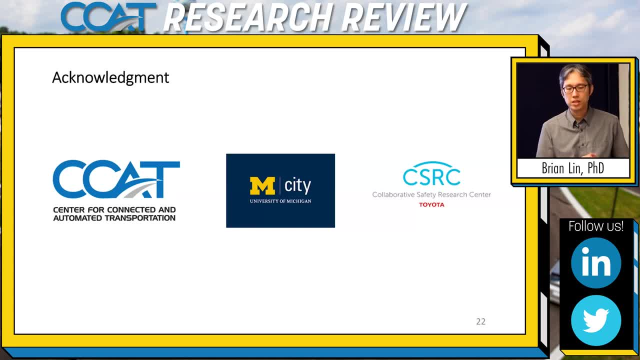 we make it consistent for the everybody's. you know the time before the lane change. So you know, since some of the some of the drivers, they may take longer time. well, they may longer time after they enter the weaving sections, but with with the different time, numbers of time, 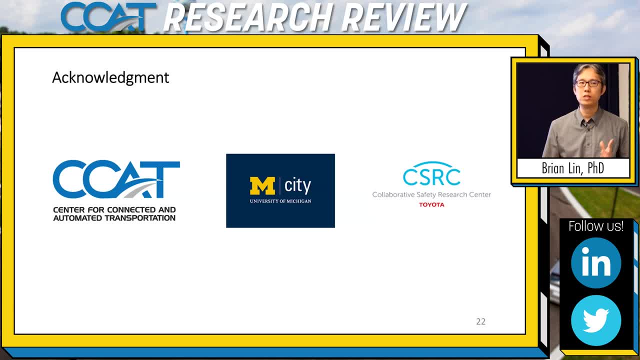 stamps. sometimes we will bias the. you know the sample we have. So we try to make it consistent across the subjects, since we have 53, we have 53 weaving sections, So we get enough data, that's so we just we don't need to, we don't need to have a wide, very wide.